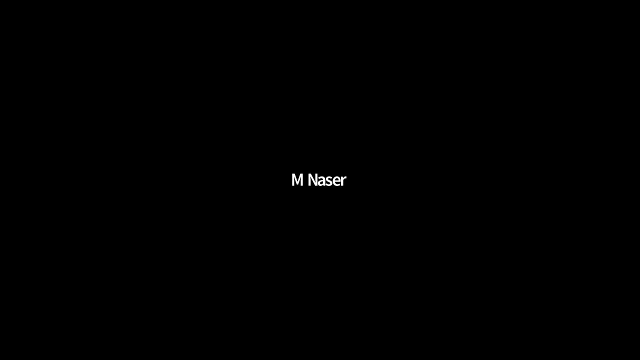 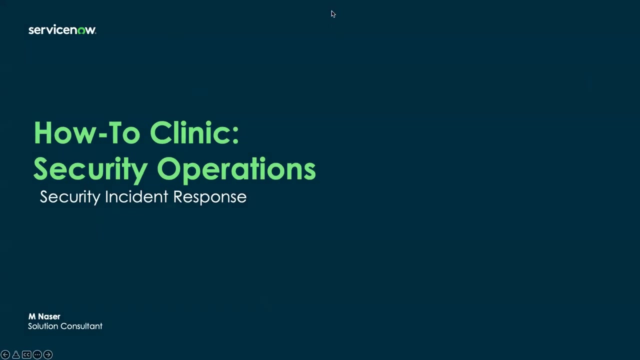 Thank you. Hello everyone, Thank you for joining us on today's webinar: How to Clinic Security Operation for Security and Service Response. My name is Mohamed Nasser and I'm going to be leading this webinar. I'm just going to give it a quick couple of minutes, just waiting. 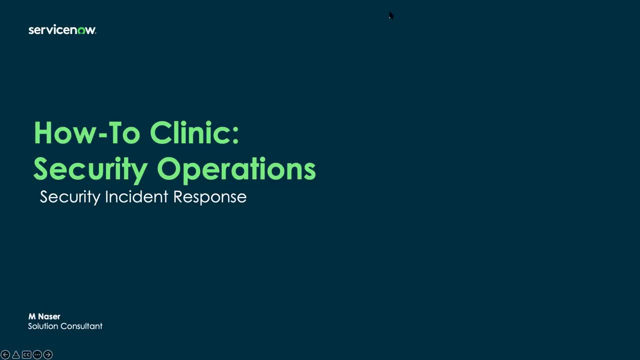 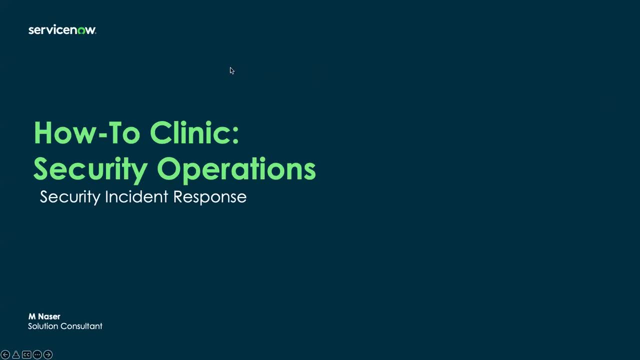 Okay, so hello everyone. My name again is Mohamed Nasser. I am a solution consultant who is specializing on the security operations offering at ServiceNow, And today I'm going to be covering the How to Clinic Security Operation for Security and Service Response. 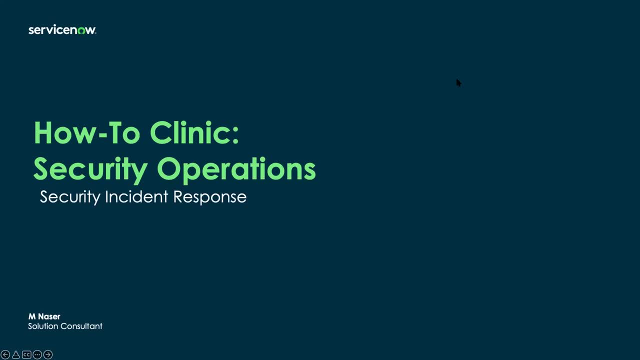 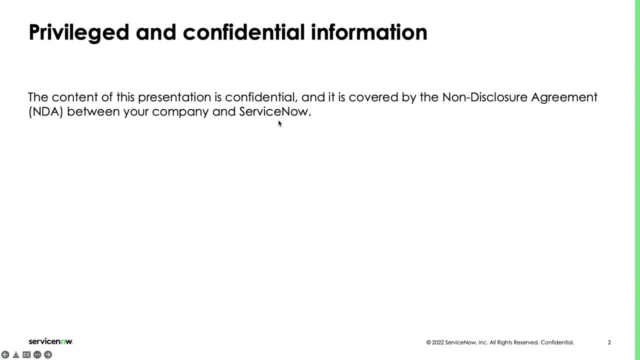 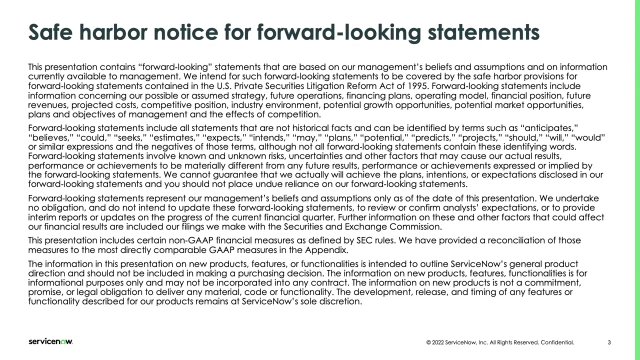 a webinar. Thank you all for joining us today. Before I get started, just a quick reminder: this is a privileged and confidential information. This is also covered by the safe harbor notice for forward-looking statements, So this presentation contains forward-looking statements that are based on our management. 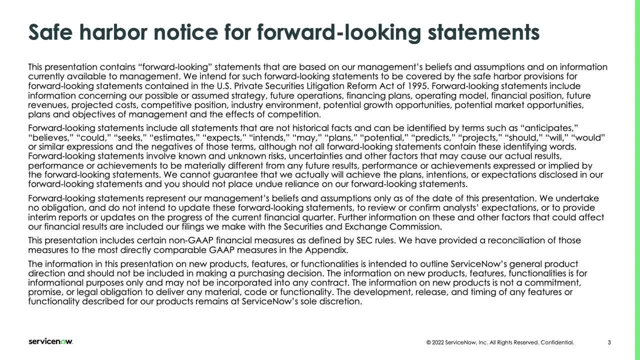 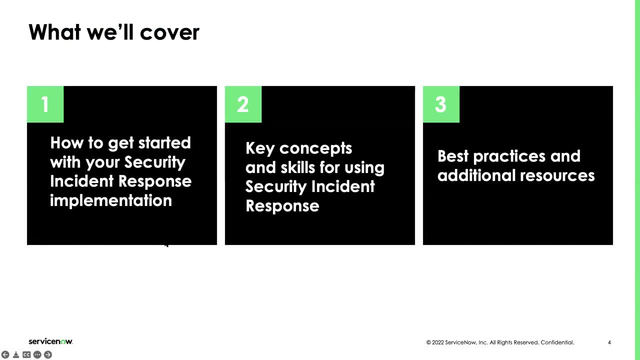 beliefs and assumptions and on information currently available to management. We intend for such forward-looking statements to be covered by the safe harbor provisions for forward-looking statements contained in the US Private Secretariat Litigation Reform Act of 1995.. So what I'll be covering today- number one- I'll be covering how to get started with your. 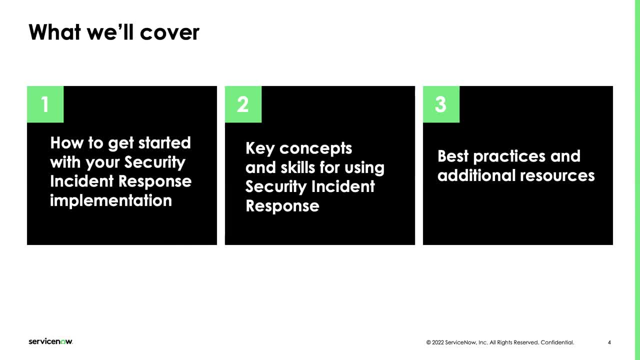 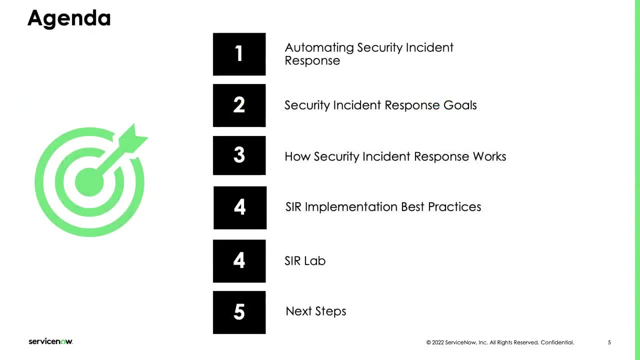 security and service response implementation, moving on to the key concepts and skills for using security and service response And, finally, the best practices and additional resources where you can find more information about security incident response. The specific agenda for today's webinar is going to be around automating security incident. 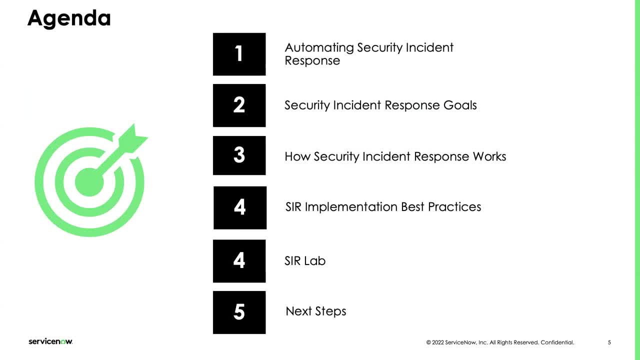 response: security incident response goals. moving on to how security incident response really works. After that, we're going to be discussing the security incident response implementation and best practices. moving on to the security incident lab, which is going to be substituted for demo for today. 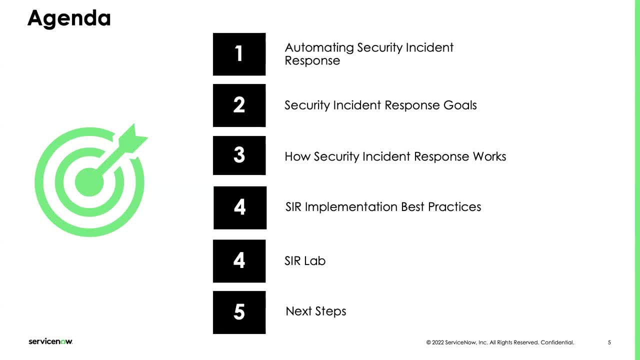 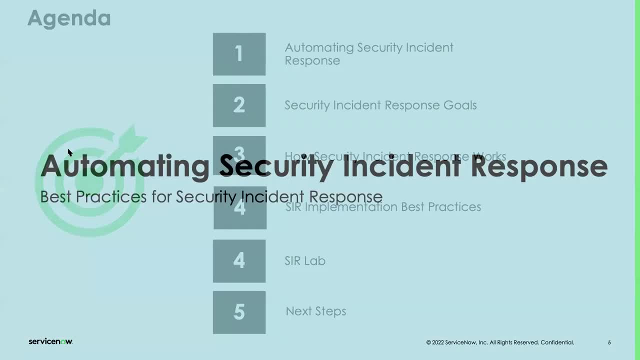 And finally, we're going to end with the next steps, where you're potentially going to be finding more information on how to get more details about security incident response. Now let's kick it in with the automating security incident response. best practices for security. 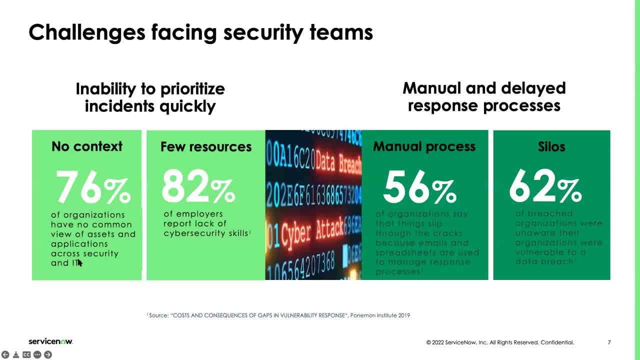 incident response. So what are the current challenges facing security teams? So the first challenge is the inability to prioritize incidents weekly and the safety of incidents. The second one is the manual and delayed response processes. So what exactly do we mean by that? 76% of all of the security incidents that we receive or common organization receive? 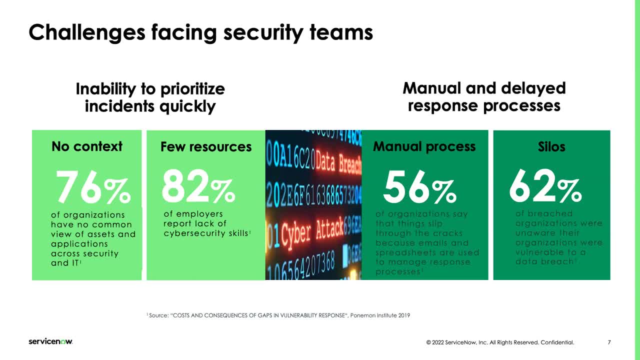 most of the time don't have specific context, So we're just being alerted with something that we don't actually understand what it means, which could potentially be a great danger, because by the time we're filling out all of these blank spaces, we could potentially be in a greater danger. 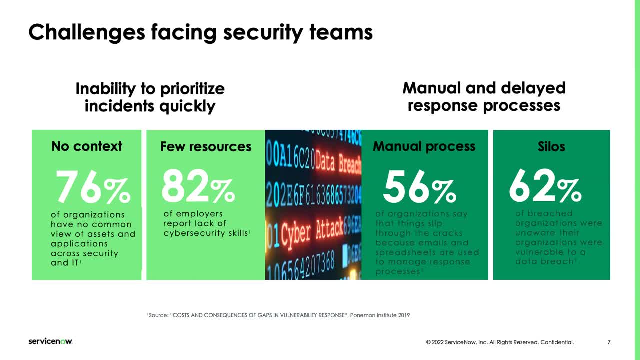 The second one is that we have few resources, So ATT&CK is one of them. There are about 52% of employees employers report lack of cyber security skills. Cyber security is a field that is continuously growing. There's definitely a bigger need for it since we move to all of the working from home things. 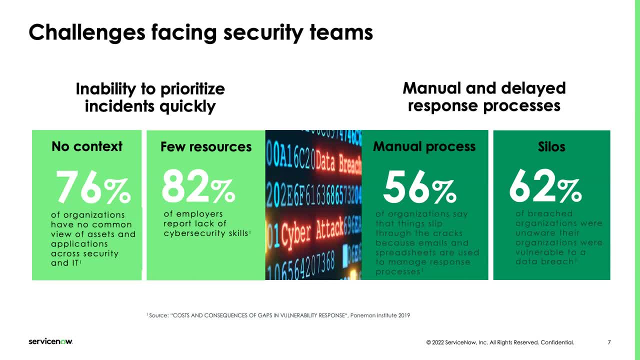 and all of the extension of digital transformation. hence why these skills are always in demand. hence why we don't have enough resources as we would like. The other part of this is the manual process that we currently rely on, so 56% of organizations. 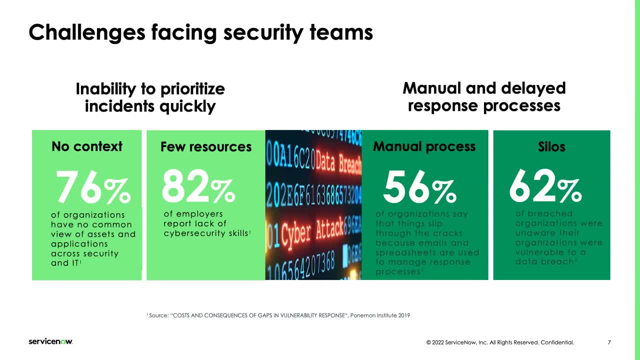 say that slip through the cracks, because emails and spreadsheets are used to manage response processes. so one of the things that we commonly face, especially working in the security world, is that we are commonly using things that are kind of outdated when we're talking security. so whether that was a spreadsheet where we basically just have a repository of all of 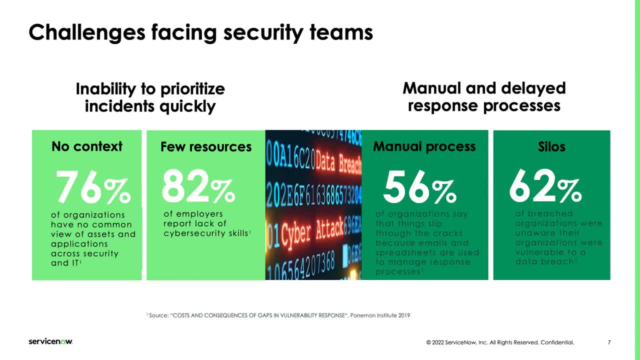 the different vulnerabilities or of all of the different security instances that we're currently working with. we're communicating through emails, which can mean that we are potentially waiting for someone to get back to us for the next step. all of that creates just a lack of time that we 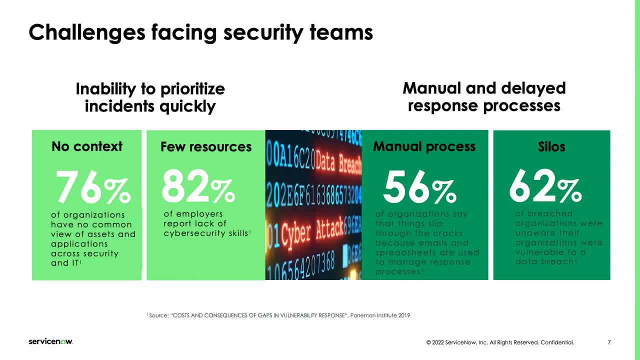 are basically wasting. the silos is already there because 60- 62 percent of breach organization were unaware their organization were vulnerable to a data breach, so silos that is naturally created between it and security teams is also one of the reasons that we could potentially be in danger. 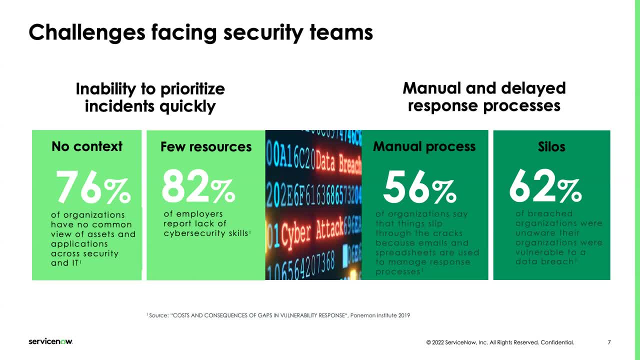 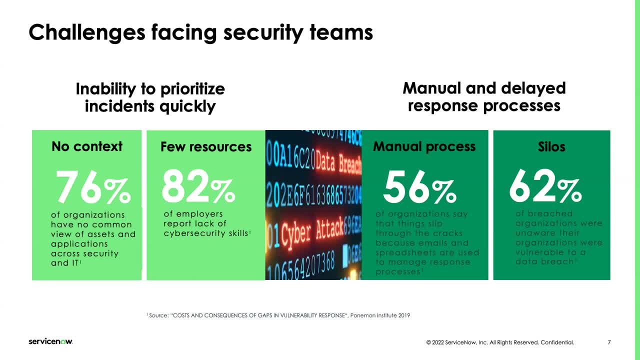 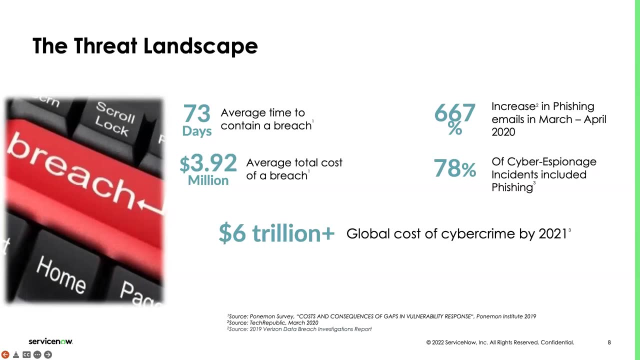 a specific action to remediate against that specific security incident or vulnerability. so hence why we are seeing this silos, because again, we're relying on all of these manual processes, so the threat lag landscape. so 73 days is the average time to contain a breach. so we find 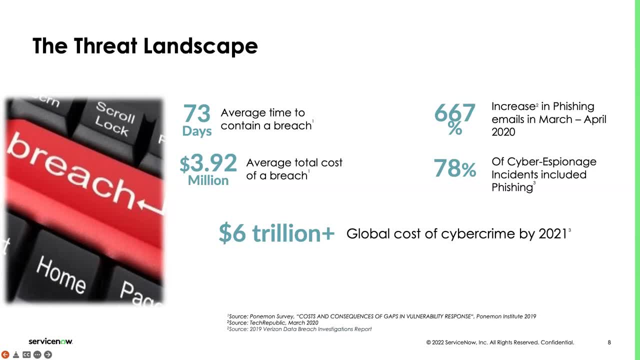 a breach. we know that exists, it takes us 73 days to actually get to that specific breach. there is a 3.92 million average total cost of a breach, and then there is a 3.92 million total cost of a breach and then there is a 3.92 million total cost of a breach. so we've always constantly here on. 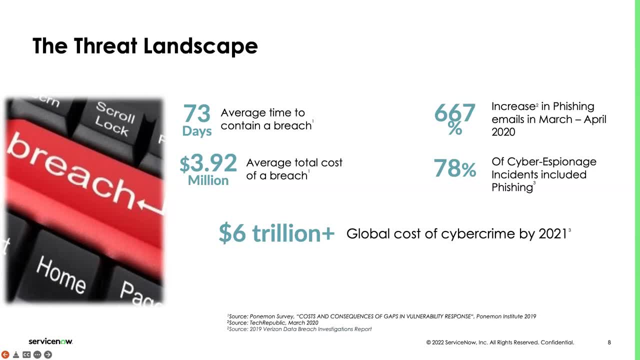 there is a 3.92 million total cost of a breach. so we've always constantly here on this on the news, this on the news. there's a new breach out there, a reputational damage that could potentially mean loss of value and either maybe a policy violation. that also means that we are up up into fines. 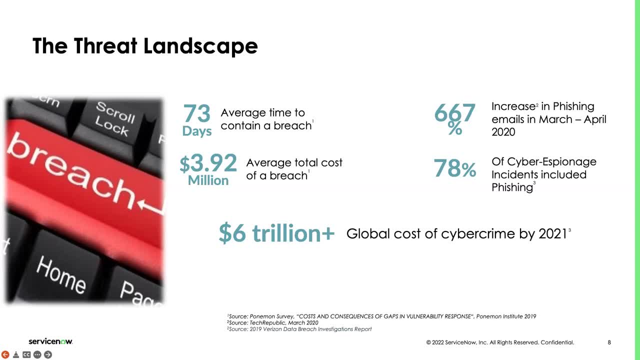 think of that nature, which costs a lot of money on the long term. so doing that or putting that investment into your cyber security, is definitely better than spending that money trying to recover from a loss that is caused because of a threat or a breach. there's a 667 percent increase on phishing emails in march through april 2020. 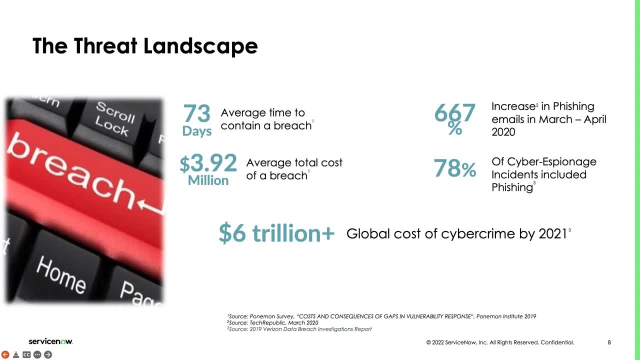 this is the time we actually moved into working from home, where a lot of hackers had seized this opportunity to create fake emails where they pretend to be who or they pretend to have more information about the covet virus or the vaccines, etc. so hence why we are seeing a crazy increase in that specific 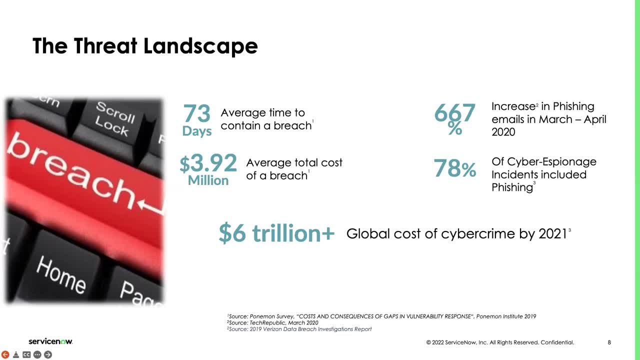 amount of time. there's also 78 of cyber espionage incidents included in fishing, so phishing is actually one of the most common security insets that we commonly see, because it's often wrapped as something that we don't think is an actual threat. there's also a six trillion dollar increase in global costs for cyber crimes by 2021. 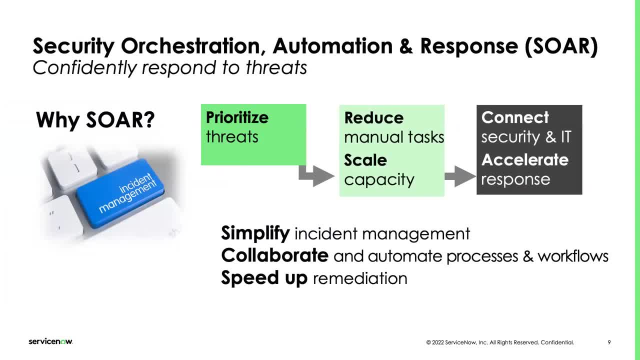 so what can we do to actually, uh, help mitigate all of these numbers? uh, this can be done to make the data that we see to help protect ourselves- so we have a great publisher- from Complian be done through security, orchestration, automation and response, or SOAR in short. So why SOAR? exactly? 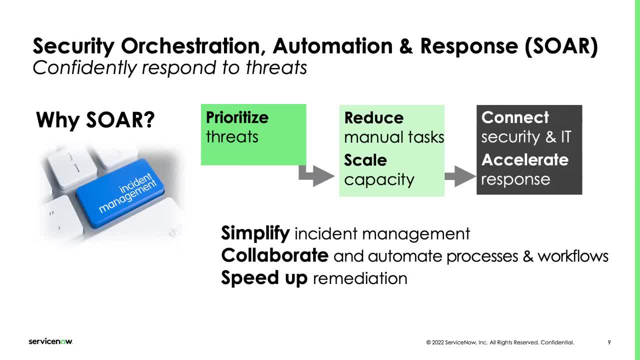 Because we want to be able to prioritize the different threats that we are receiving in our environment. We can also use that to reduce the manual task scale the capacity of our own employees. We also use that into connecting security and IT and cancelling the silos that. 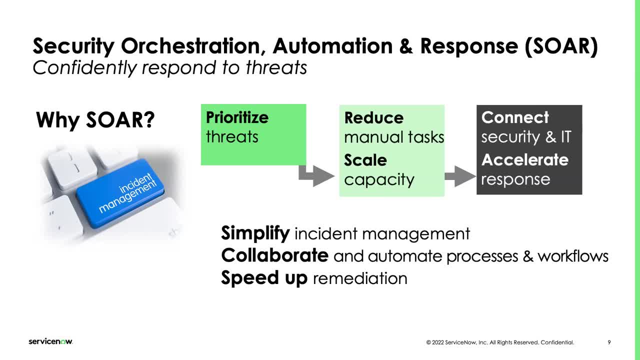 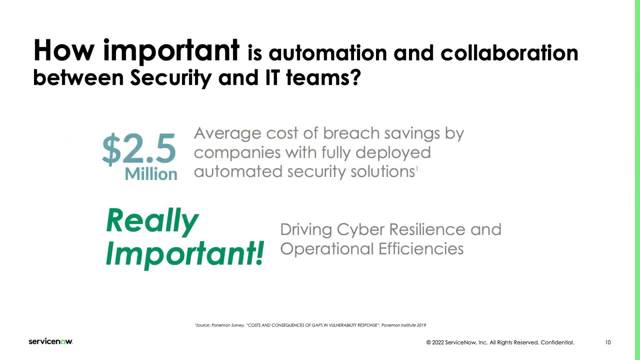 is created and, in result, we're able to accelerate the response or the response tasks that are associated, whether that means that the security teams need to do something or the IT needs to do another thing. So how important is automation and collaboration between security and IT teams? There is a $2.5 million average cost of bridge saving by companies with 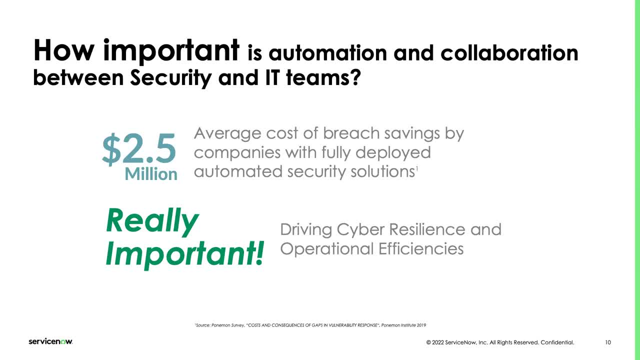 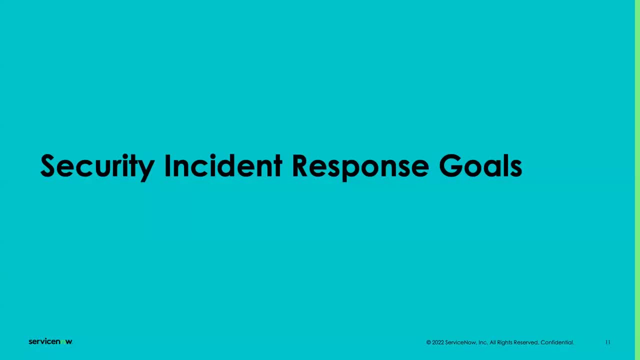 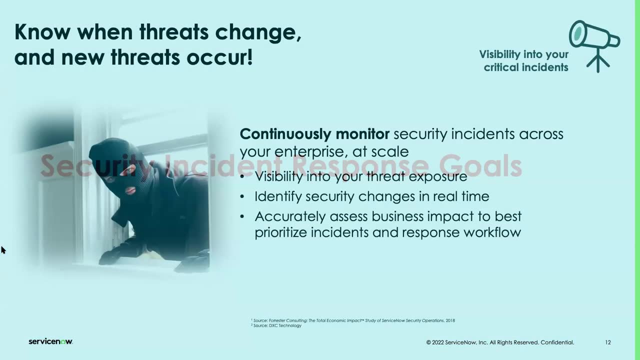 fully deployed automated security solutions and it's really important because it drives cyber resilience and operational efficiency. So what is the specific goals of security incident response? So we want to know when threats change and new threats occur. So we want to be able to continuously monitor our environment. So security incident across your enterprise at scale. 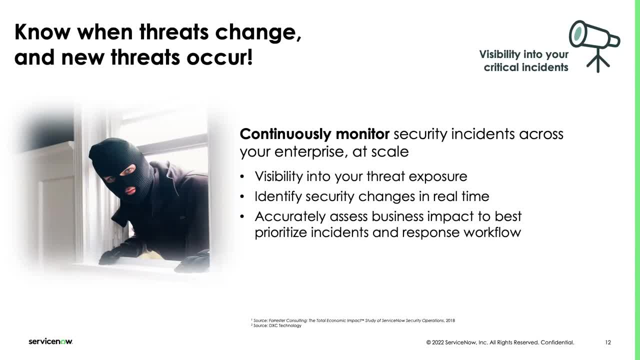 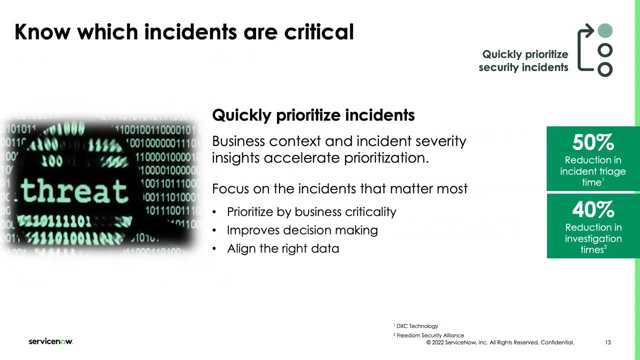 we're going to be providing you with visibility into your threat exposure. We're going to help you identify security changes in real time and accurately assess business impact to best prioritize your security risk. So we're going to be providing you with visibility into your the incidents and response workflow. We also want to know which incidents are critical. 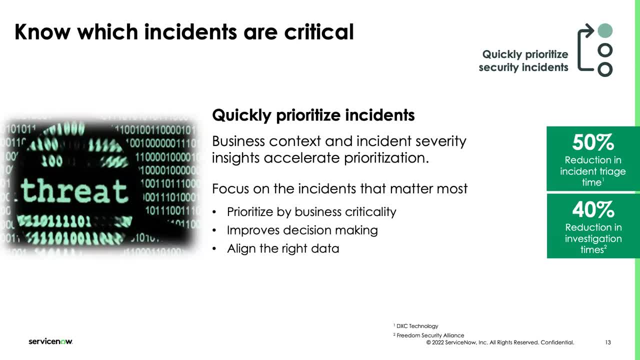 so quickly prioritize incidents. So business context and incident severity insight accelerate prioritization. So we want to focus on the incidents that matter most, with prioritizing by business criticality, improve the decision making and align the right data. Now having a source solution means that we are also going to be able to stay ahead of. 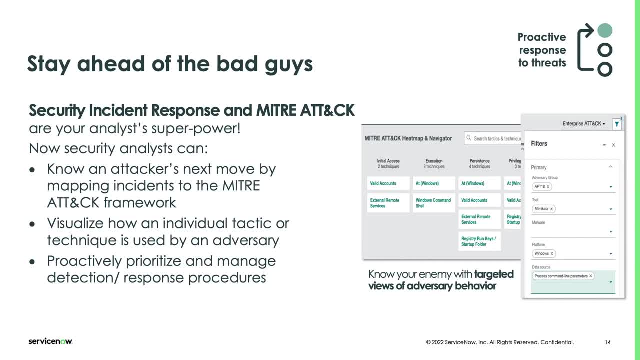 the bad guys. What I mean by that is that security incident response and MITRE ATT&CK. one of the integrations that we have on the ServiceNow platform is the ability to integrate with MITRE ATT&CK, which could help us into the investigation process of specific security. 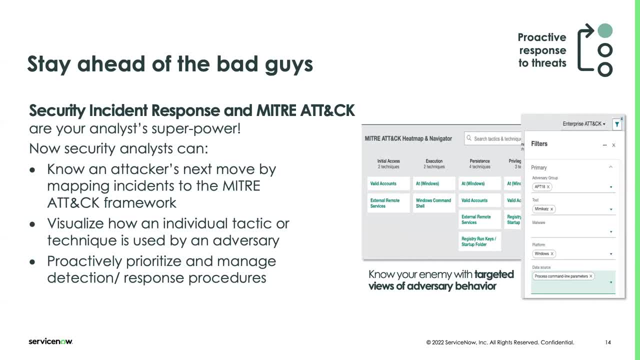 incidents or vulnerabilities that can look a bit deceiving because of how small they are, when in fact they are part of a bigger tactic that can potentially be a greater danger. So, being always aware of what a specific attack means, or what a specific vulnerability means, or the specific steps that the hacker might take into 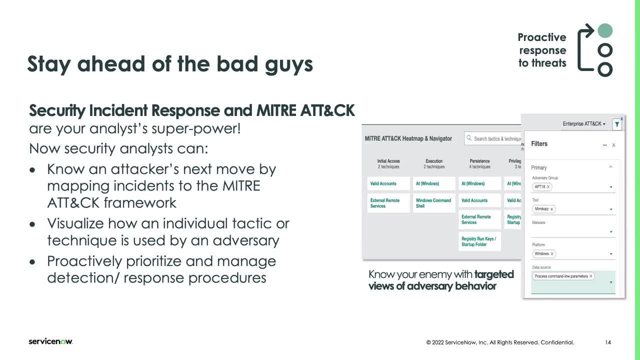 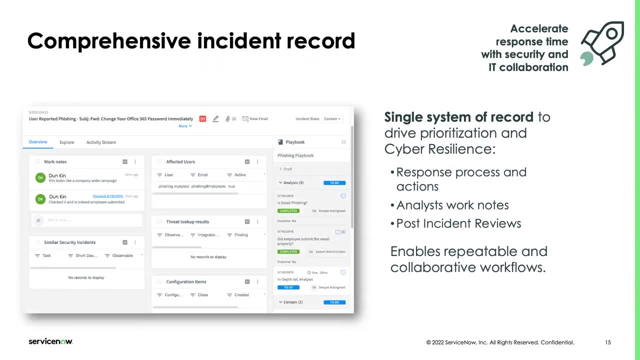 actually gaining access to your environment by utilizing the information of MITRE ATT&CK is critically important in this case. The comprehensive incident record is going to give us a single pane of glass where we're going to be basically looking at all of the information that is available to us on the security incident. So, as you can see, on the 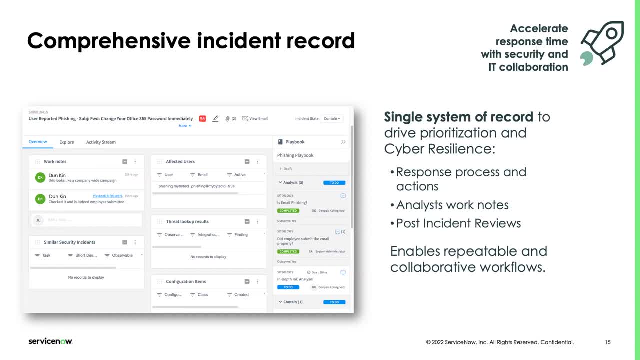 screen. it's going to give us a single pane of glass where we're going to be basically looking at all of the information that is available to us on the security incident. So, as you can see on the screen right now- and this is also something that you're going to be seeing once we move to the demo portion- 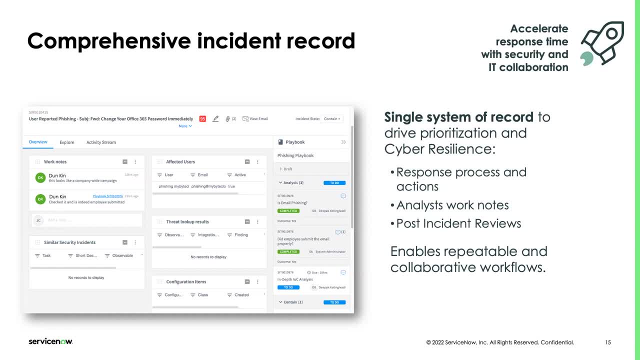 is that we're able to see more information about the specific security incident. The work notes that is within the different teams, so either the IT team or the security team- both of them are communicating on the same page, So canceling all of the need for emails and Slack. 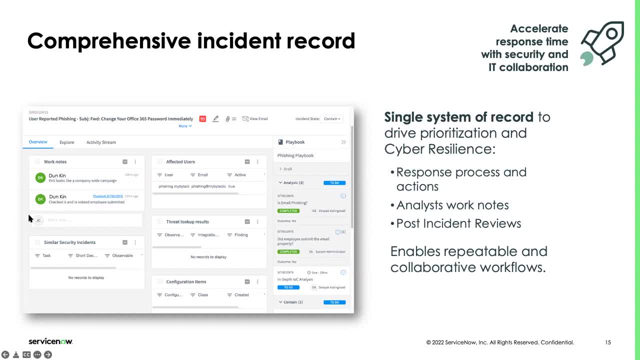 teams, etc. We can see who are the affected users on all of these different security incidents, whether there are similar security incidents or not. On top of that, we are utilizing the playbook, which gives us basically a step-by-step approach into how we should be handling. 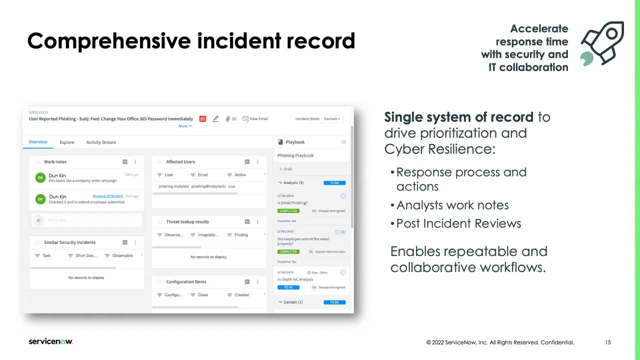 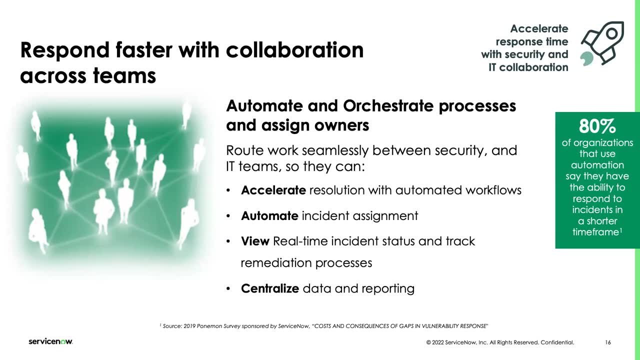 a specific security incident from start all the way until it's actually contained. We also want to be able to respond faster with collaboration across the team. So, as I mentioned previously, having a single pane of glass is definitely going to help us into accelerating the resolution through either the single pane where we are communicating with each other. 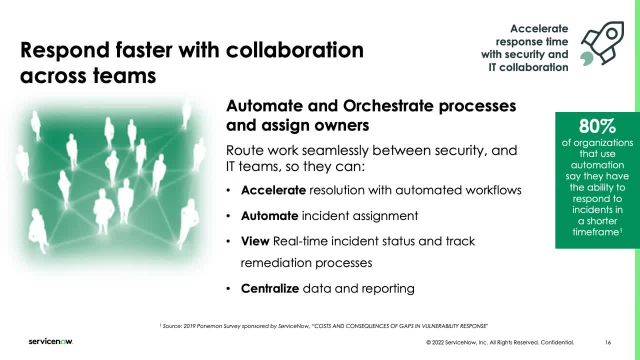 or also utilizing the magic of ServiceNow, which is within our workflows, where we can basically automate a bunch of different steps that usually are done manually. We can do that through automating the incident assignment. We can view the real-time incident status and track the remediation process. 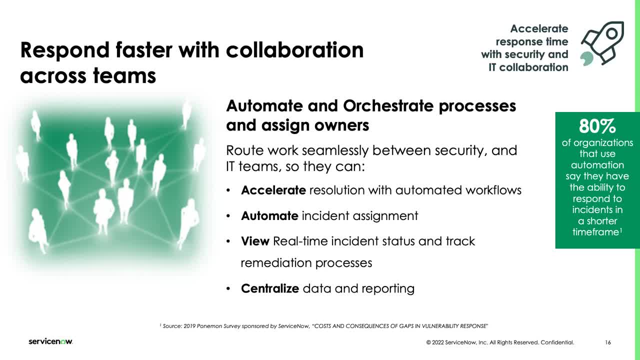 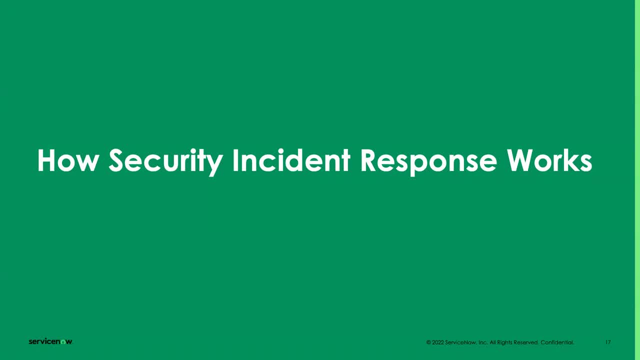 And all of that is through the centralized data allocation. So we've seen why security incident response is important and how ServiceNow is going to be basically working. When we open the suite, we can use the Druidrup server to deal with the working toward achieving all of the prioritization. 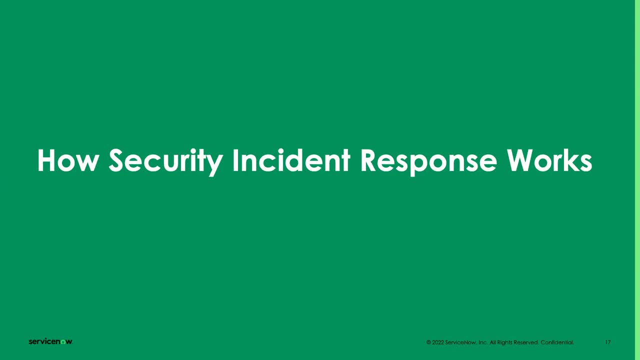 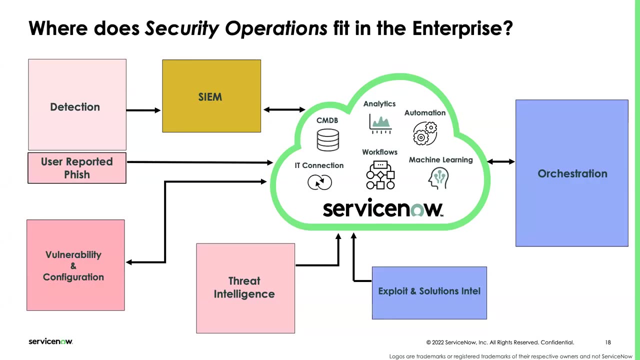 and centralization of your efforts, but how security incident response actually works and where does it fit into your enterprise? So the first thing is: where does security operation fit into an enterprise? As we are all aware, there are a bunch of different services that we currently use for our cybersecurity efforts. 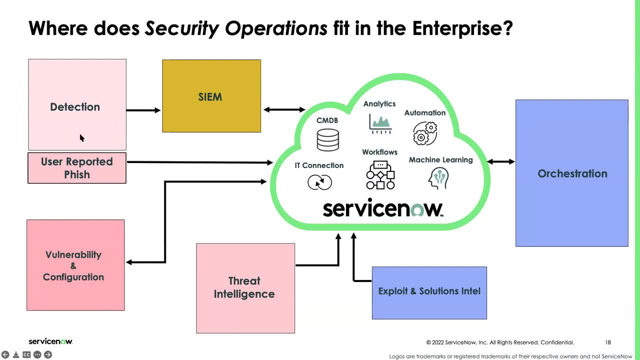 Some of these devices or services are done for detection, Some are just simple CMs, Some are vulnerability scanner and configuration scanners, And all of this information are going to be ingested into the ServiceNow platform along with any user submitted one, whether that was for a user reported phish. 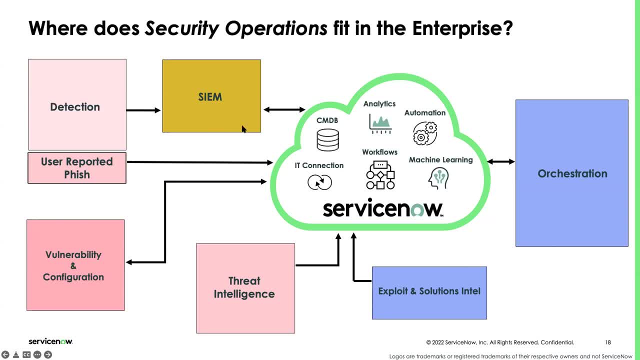 or anything of that nature, After they are ingested into ServiceNow. we're going to be utilizing the CMDB, if it exists or if it's in a mature place, where we're going to take all of the information, match it across our CIs. 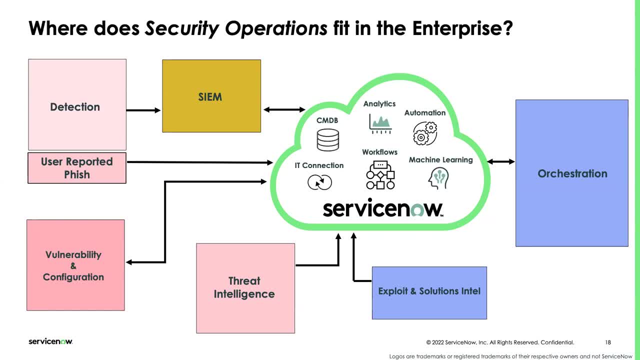 and see how critical they are to our operation. Based on that, we're going to be determining the priority of these different alerts that we've ingested, After ingesting them, and categorizing them. so if it's a phishing attempt, then the workflow for phishing is automatically gonna kick in. 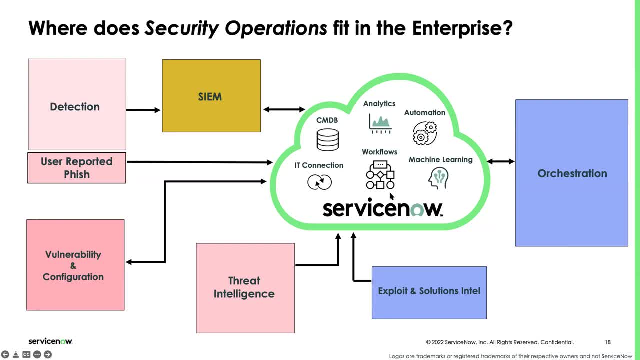 If it's a vulnerability, then the vulnerability workflow is automatically gonna kick in, which can mean that if there are any specific tasks that we would like to be automated, like, for example, curating the host until we're done with the investigation, or deleting the email. 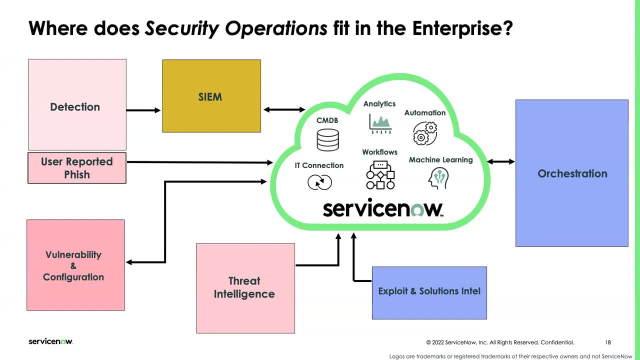 if it contains a specific hash file that we know that is a malware, then we can automatically take care of that through the automation part within the workflow. We can also utilize the information of threat intelligence and exploit and solution intel to help us in our investigation process. 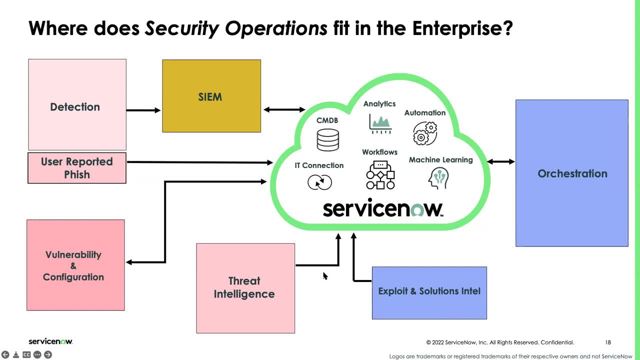 So, again, I mentioned the example of the hash file. How did we determine if that specific hash file is in fact malicious? That can be done through the threat intelligence integration that we have with services like CrowdStrike or VirusTotal, where you can automatically scan the hash file. 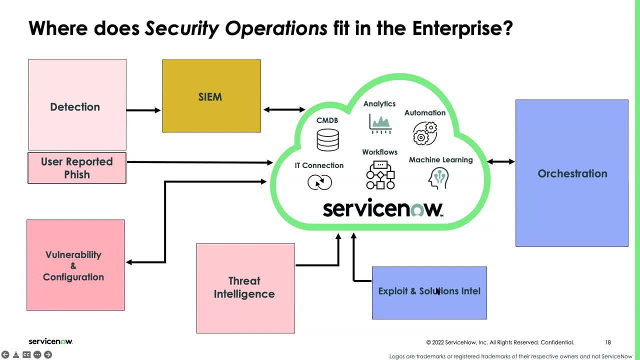 or the IP to give you the findings on it, The exploit and solution. intel can help us into determining what is the appropriate solution, based on maybe a vendor fix or something of that nature. Machine learning is where we kinda are going to be utilizing information like ticket assignments. 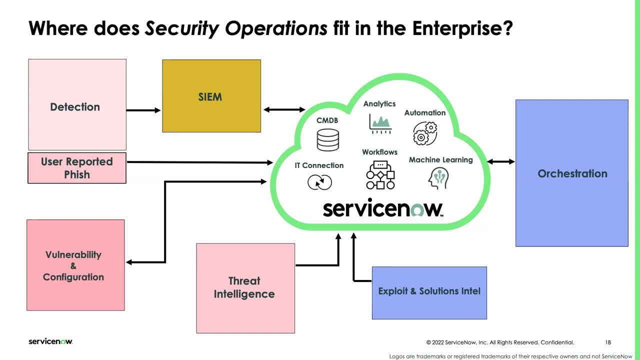 or incident assignments. So if we receive a specific incident that is existing, maybe in San Diego, then the machine learning part is gonna take that incident and assign it to an individual who is located in San Diego over assigning it to someone who is located on the East Coast. 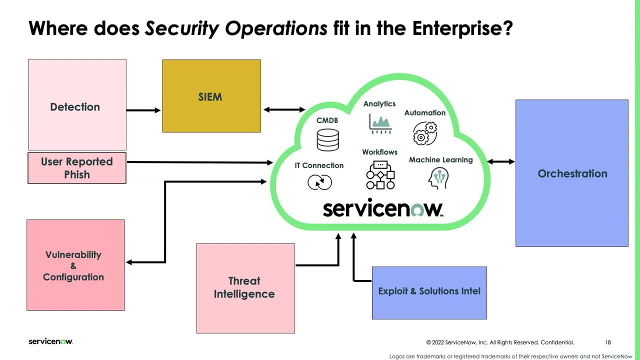 because just of the time difference. So this is something where we can utilize machine learning to help us assigning the different incidents. The orchestration part is basically where we are able to initiate a two method communication between the ServiceNow platform and any of the different services. 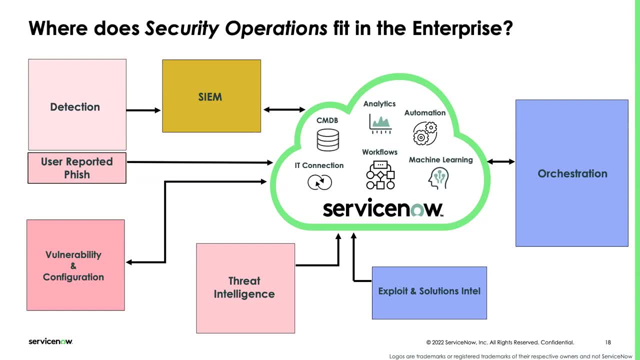 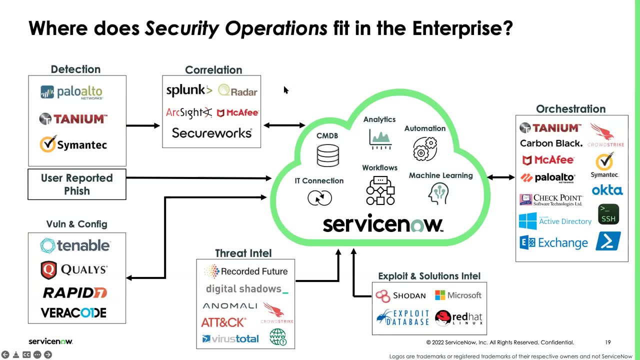 that can perform actions in our configuration items. So in the example of isolating the host or quarantining it, then we can leverage the orchestration tools to do all that. Now this slide actually looks a bit different and might help you understand the concept a little bit more. 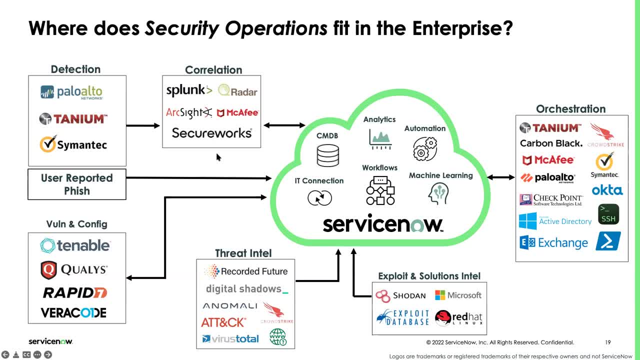 The reason for that is that it gives you an example of all of the different devices and services that can be integrated with ServiceNow. So the detection we can integrate with Palo Alto, Tanium, Symantec, invulnerability and configuration we can integrate with Tenable, Qualys, Rapid7,. 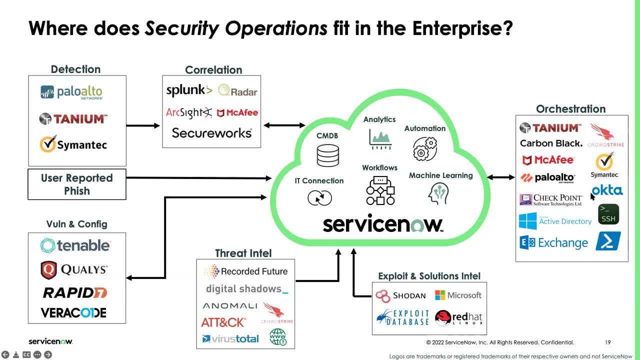 Threat Intelligence, VirusTotal, CrowdStrike, Orchestration, CrowdStrike, McAfee, Palo Alto, Explosion Instruction, Intel, Microsoft. So, again, this is just an example of all of the different integrations that can be done with ServiceNow. 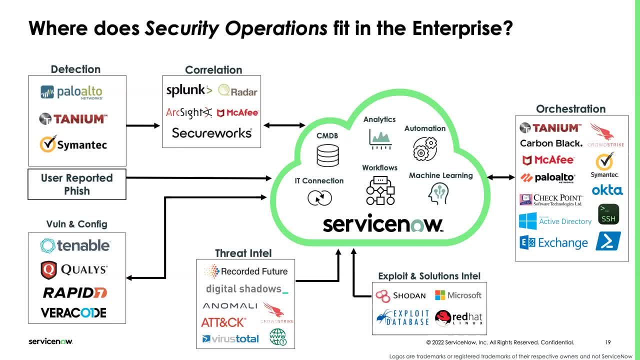 or on the ServiceNow security incident response solution For a full list of all of the different integration. you can visit storageservicenowcom to see if the device or service that you're using has a prebuilt integration. I'm gonna be covering how we can. 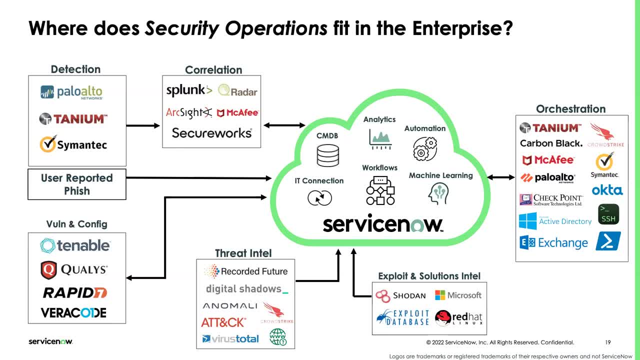 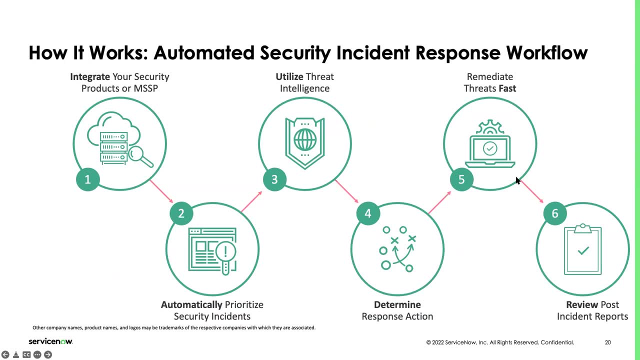 see what sort of integration is available to us. all of that on the next slide. So, again, this is just an example, So how it works: automated security response workflow. So, as I mentioned, one of the ways, or the most important thing, that we need to focus on. 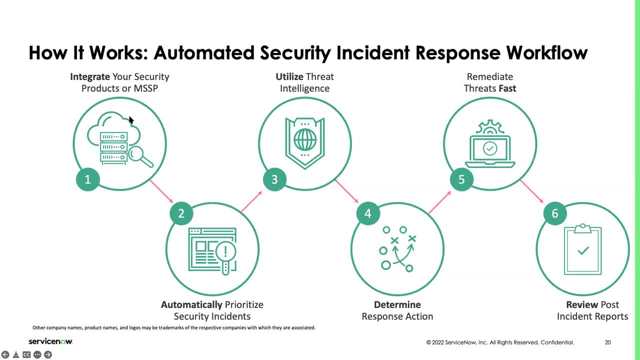 is integrating your security product or MSSP, So we rely on the third party integration into the platform, whether that was from Splunk, Radar, LogRhythm, et cetera. We're basically are going to be getting information that is going to be categorized as a threat. 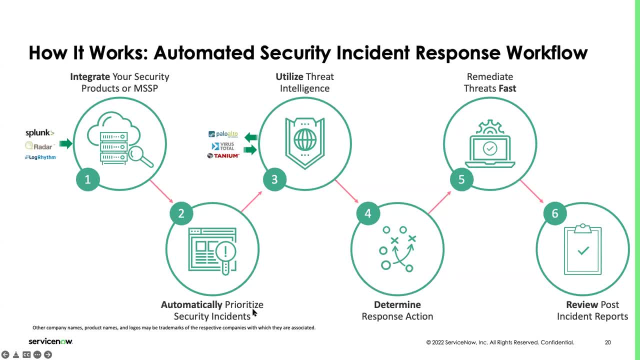 After that, we automatically prioritize the security incident based on the information in our CMDB or based on our own implementation rules. We utilize Threat Intelligence into also determining the criticality or the business impact of these different threat alerts. After that, we determine the appropriate response action. 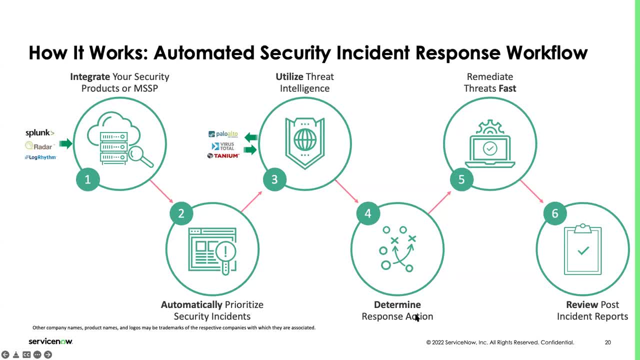 whether that was through the different playbooks that we have built ourselves or integrated from different services, We assign the different tasks to the appropriate individuals and from that we are going to be able to remediate the threat faster. And throughout this entire process, 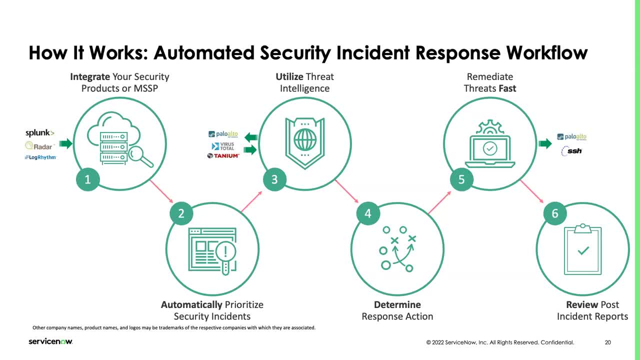 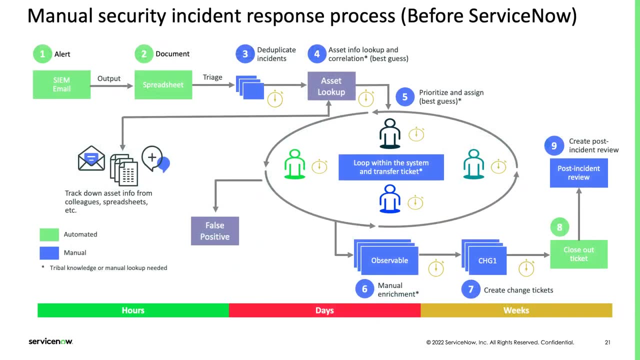 the review and post incident response are automatically available to us. These can also be leveraged into you know, the you know, to creating future playbooks or just creating lesson learned exercise or something of that nature. Just to give you a quick visualization. 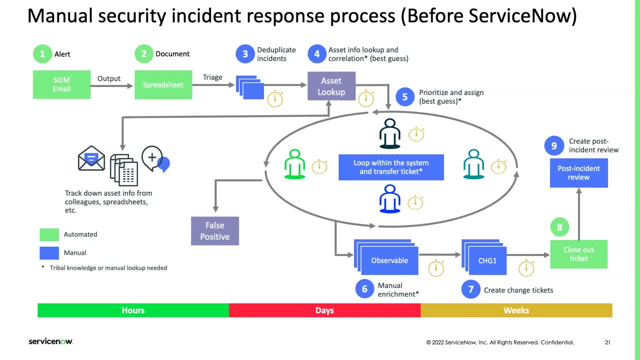 of the manual security incident response process before implementing ServiceNow. So, as you can see, we have a bunch of different automated steps that are working hand in hand with the manual steps. We can see how the manual ones are actually stretching out the response time from hours to days to weeks. 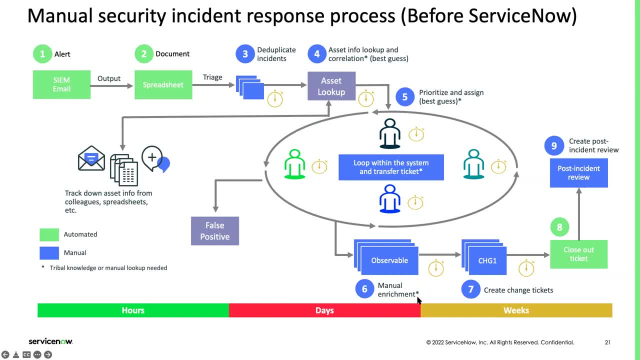 And this is just because we are waiting for a response from a specific individual, or we have to go ahead and perform a specific task manually, Hence why we are seeing that stretch of time. Now, how would that look after implementing something like ServiceNow? 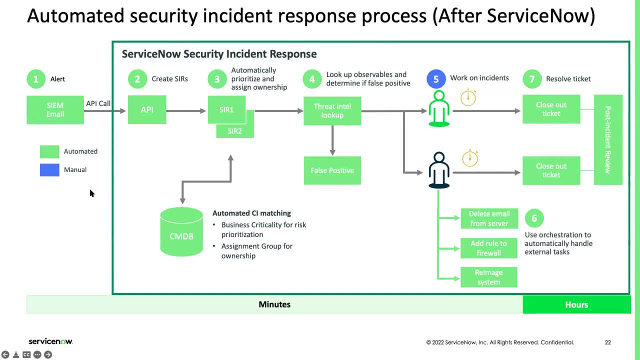 We can see how most of the manual steps are actually now automated, So we are able to cut down the response time from all of these weeks or days into just a matter of minutes and hours, depending on the maintenance window and whether we can actually perform an action or not. 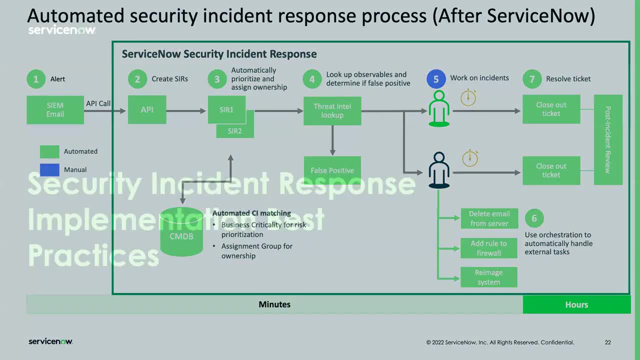 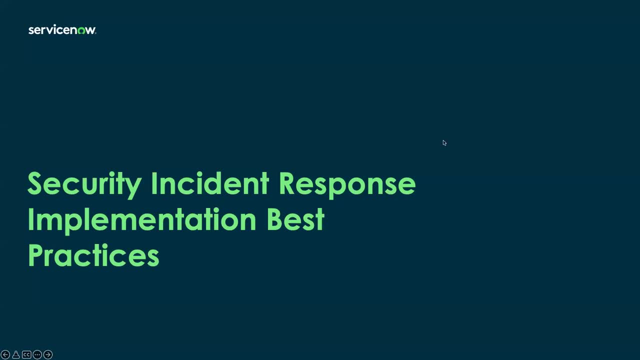 Again, if you have any questions, please feel free to utilize the Q&A part, and I'm going to be answering that toward the end of this webinar. Now, security incident response: implementation and best practices. Security incident response accelerator: look for your integration. 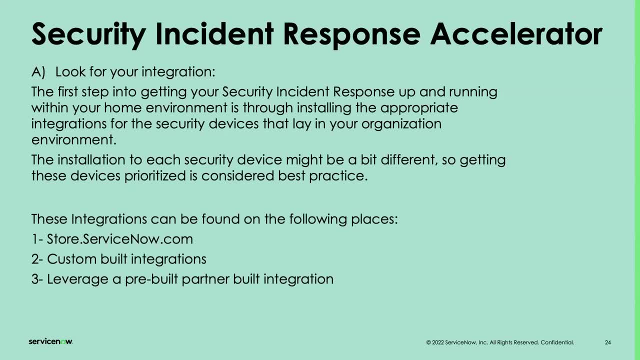 So the first step into getting your security incident response up and running within your home environment is through installing the appropriate integration for the security devices that lay in your organization environment. So the installation to each security device might be a bit different. So getting these devices prior to rise. 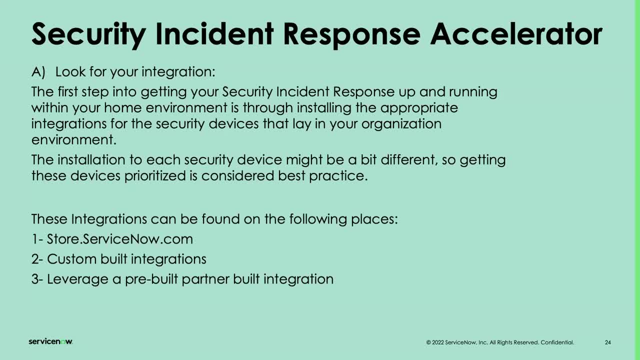 is considered best practice. So what I mean by that is that we need to understand what we currently have, or what are the different devices or services that we currently have. First step would be to go to the ServiceNow store, which is storeservicenowcom. 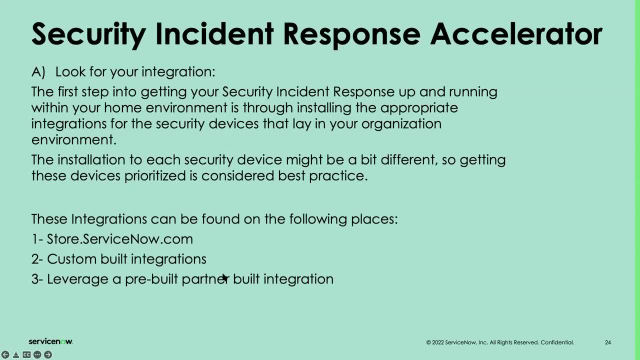 to check to see if that integration is already pre-built. As you know, ServiceNow has great connection with most of the security vendors out there. Hence we have a lot of already pre-built integration available in our store Now in some rare cases. 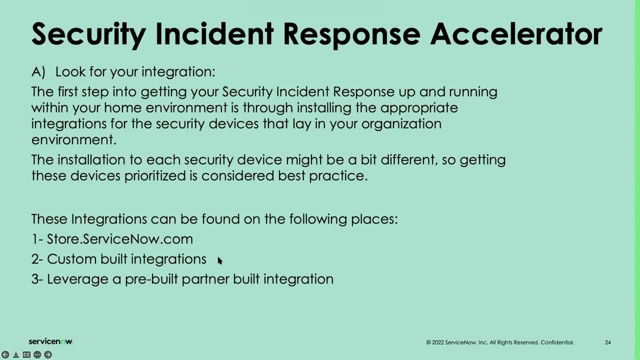 you might not find this integration. So one of the routes that you can take is that you can custom build that integration. So if the device or service that you currently have has an open API, then you can definitely leverage that into building that custom integration. 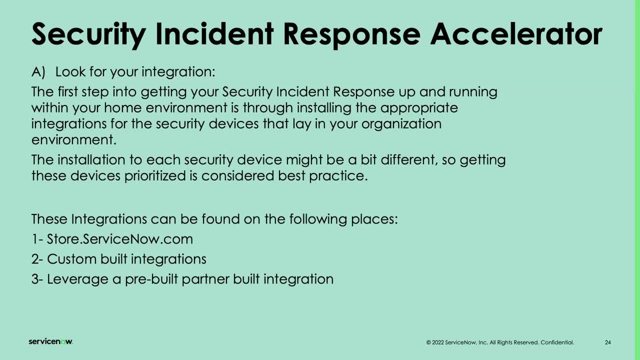 or you can leverage a pre-built partner build integration. So some open source services like the one I mentioned, or some open source devices or services don't have an integration built for them. You don't wanna actually take the burden of building that integration yourself. 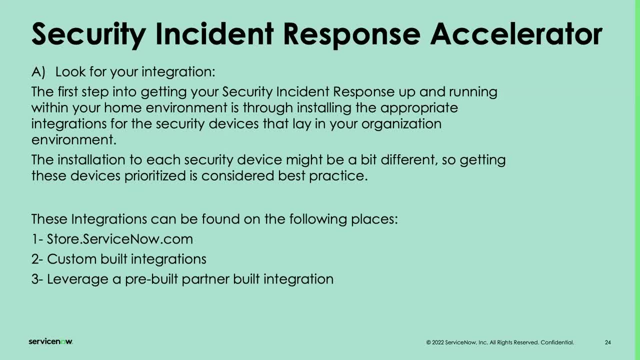 Then you can leverage one of the partners that have implemented ServiceNow in the past where they have built that integration, to just take the information that they've built in the past and implement it in your environment. And having a partner or finding the suitable partner. 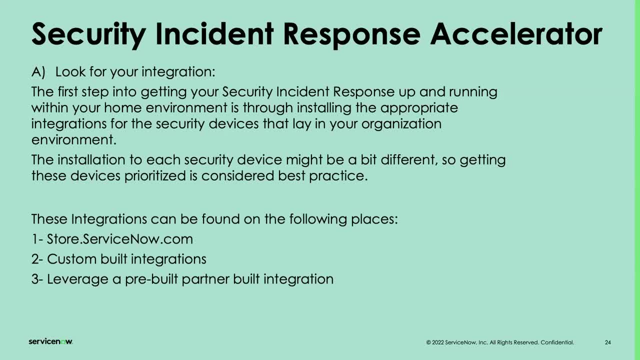 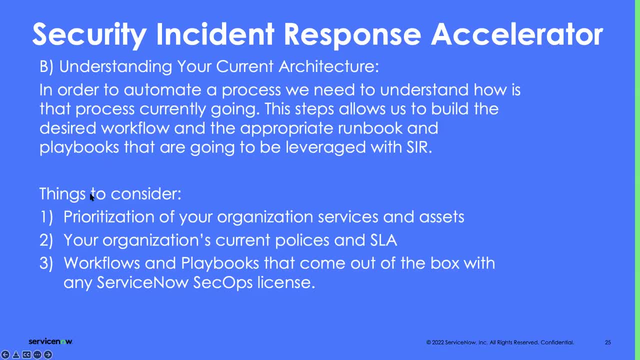 is definitely something that we strongly recommend, which is something I'm also going to be covering towards the end of today's webinar. So the next part of the Security Insider Response Accelerator would be to understand your current architecture. So, in order to automate the process, 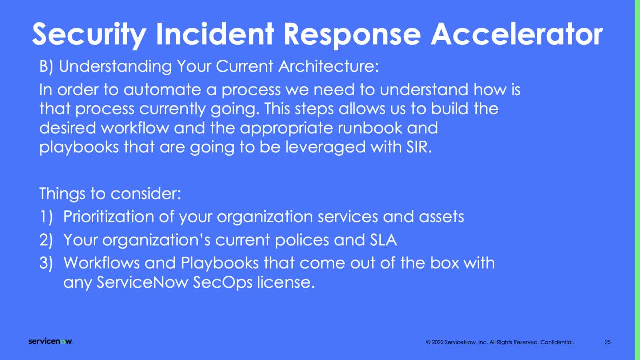 we need to understand how that process currently is going. So this steps allows us to build the desired workflow and the appropriate runbooks and playbooks that are going to be leveraged with Security Insider Response. So what are the things that we should consider in this case? 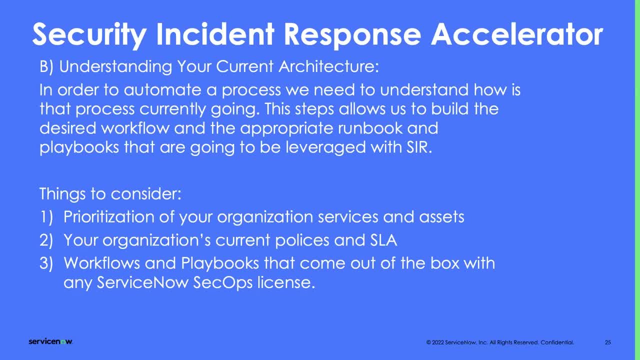 Number one is the prioritization of your organization services and assets. So we need to know what is the important asset to you and what is the services that are considered critical to your operation. So these are automatically going to get the prioritization if they receive a security alert or something on them. 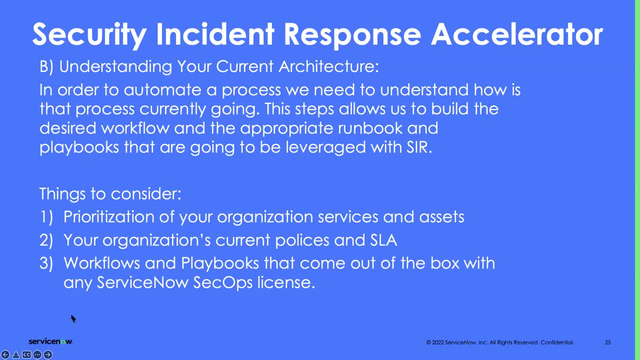 Then you need to understand your organization's current policies and SLA. So we always want to be aware if there is a policy that we might not be in compliance with by not performing a specific action on it, or if there is an SLA that might be preached. 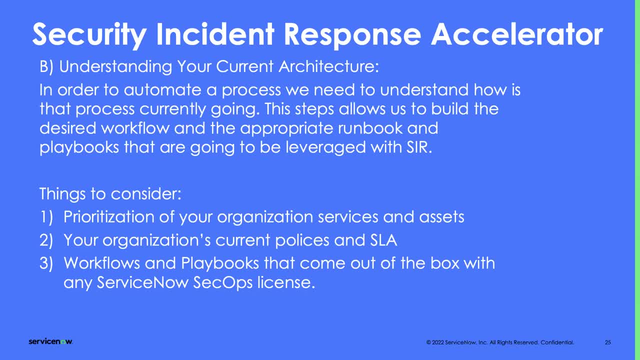 if we don't resolve an incident in the appropriate time. So having that in mind when we are building our workflow is definitely going to be beneficial. Number three is workflows and playbooks that come out of the box with any of the ServiceNow SecOps licenses. 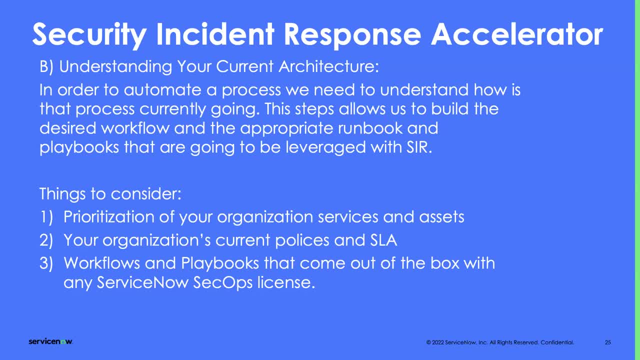 So some of the playbooks that come out of the box in ServiceNow, like the malware or the phishing attempt, these can be ready to run straight out of the box, So you can just take them, integrate them into your environment, modify the tasks that come out of the box. 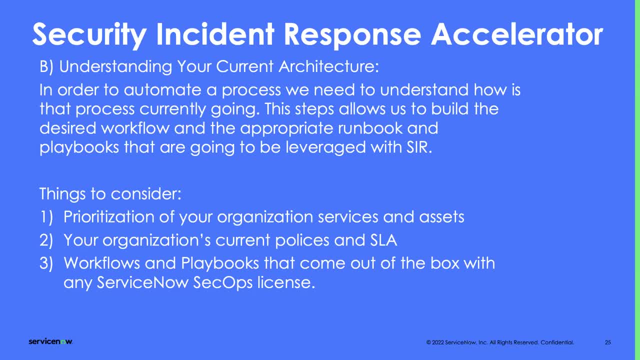 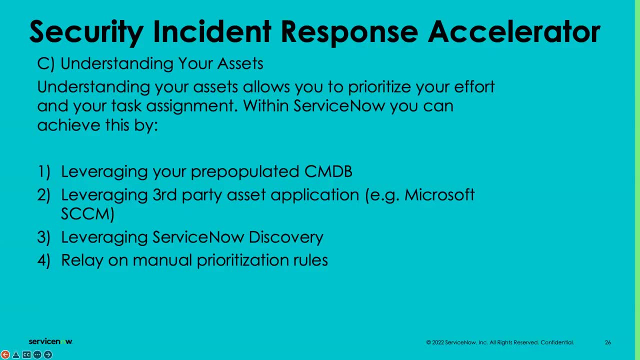 So fit your own needs, and then you are ready to run with them. Now, lastly, would be understanding your assets. So understanding your assets allows you to prioritize your efforts and your task assignment. Within ServiceNow, you can achieve this by three. 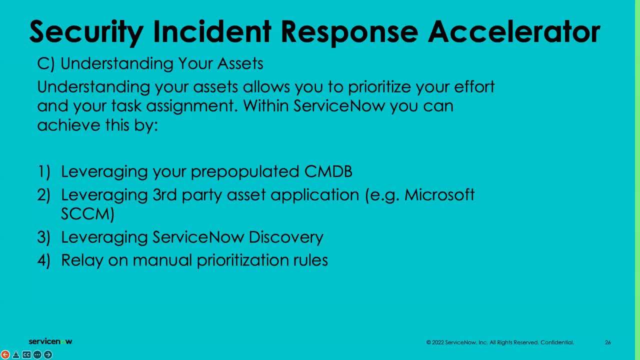 or four ways. Number one: leveraging your pre-populated CMDB. So if you have a CMDB into place, this is great. This means that you already are aware of what needs to be prioritized, when and what is critical to your. 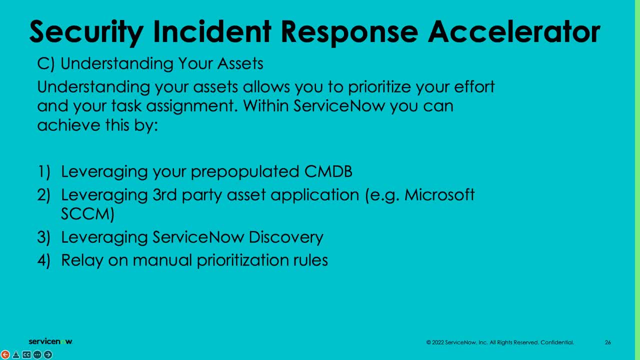 operations and this is how we get to determine the prioritization of the different threats that we receive on your different CIs. We can also leverage third-party asset application like Microsoft SSM, so SCCM, which can help us into again. 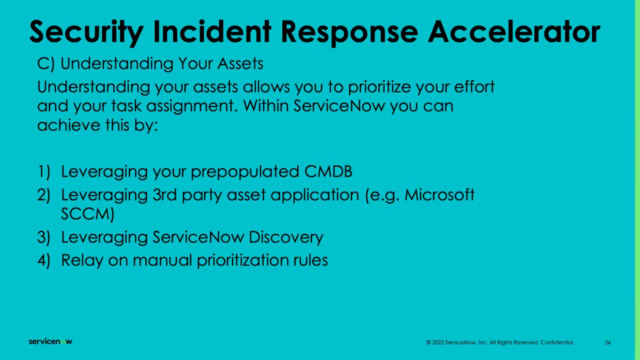 prioritizing the CIs that you have within your environment. Now, if we don't have a CMDB into place and we are not leveraging a third party, but we are interested in building one, then we can leverage the ServiceNow discovery. 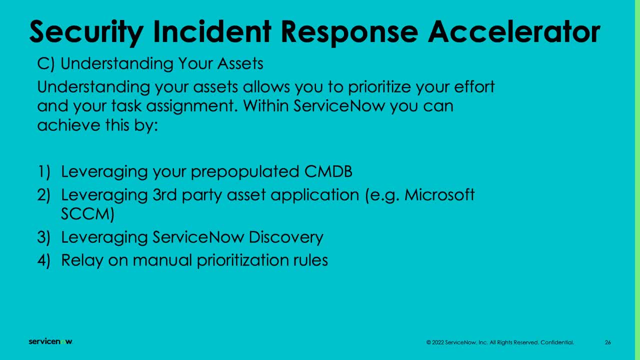 So this is an a point that you can bring up with your sales team, which can take you to the ITOM team to talk to you about discovery, which is a method that ServiceNow uses into building or pre-populating your CMDB. 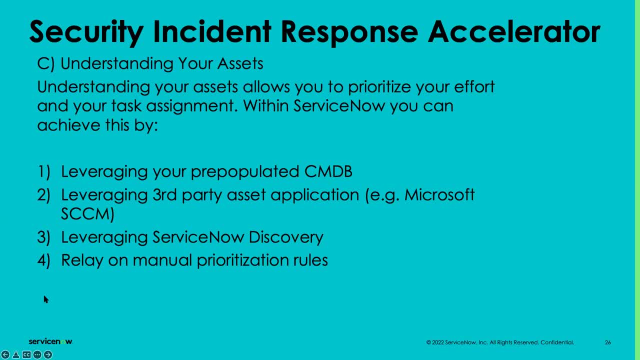 And, lastly, relying on the manual prioritization rules. So, as I mentioned in the presentation, we can rely on specific rules that we put into place, like saying, for example, if the finance department gets an alert, this gets high priority than the cafeteria. 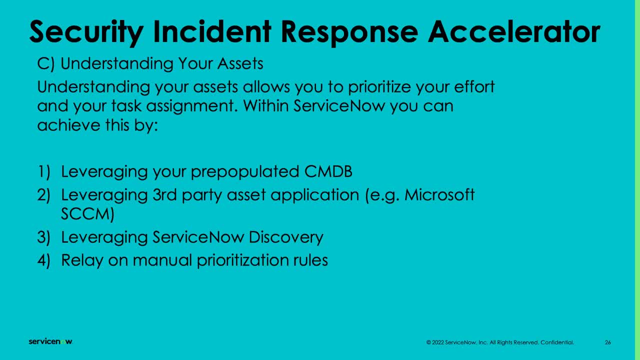 or if the CISO received an alert on this computer or a threat on the computer, this gets higher priority than just a normal employee. So all of that can also be fed into the, the platform to put into mind when we are prioritizing the different threats. 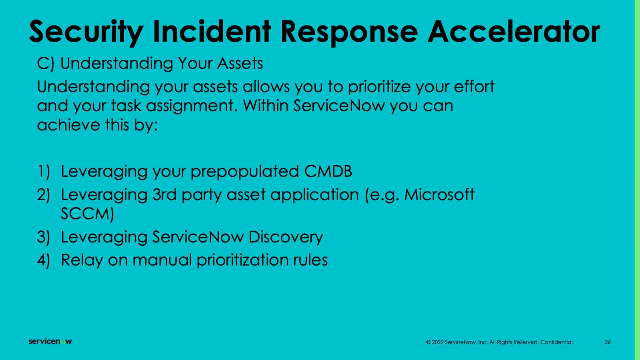 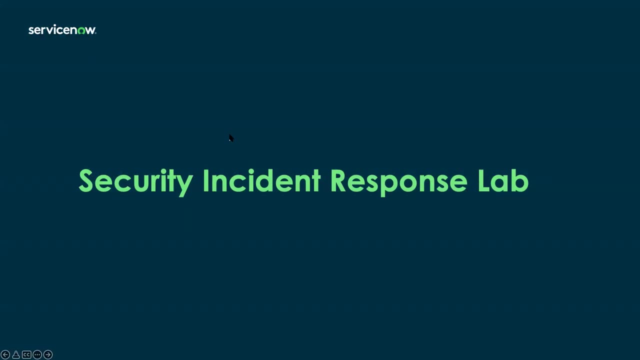 and alerts that we're receiving. We can also use a combination of the information on the CMDB and these specific implementation rules when we are determining the criticality or the risk within these different security instruments. Now I'm going to be pausing here for a quick second. 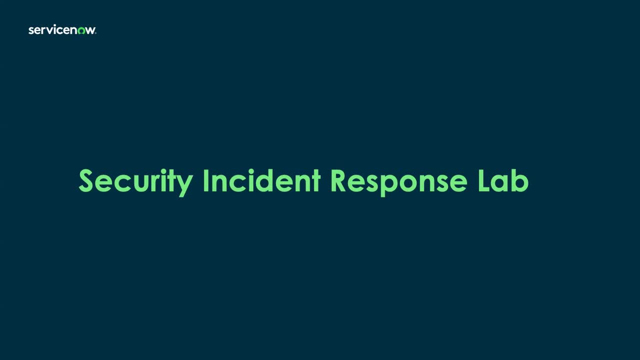 to move into the instance to actually perform a quick demo on what security incident response really means and how that would look like. Again, if you have any questions, please feel free to utilize the Q&A. If you have any further questions, please reach out via the Q&A section. 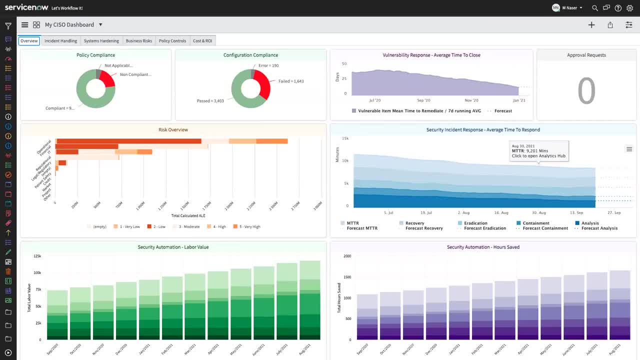 or let us know via the Q&A section or email with any questions and we'll get back to you in just a few minutes. Thank you, Thank you, Thank you. Okay, So over here we're going to take a look at the CISO dashboard. 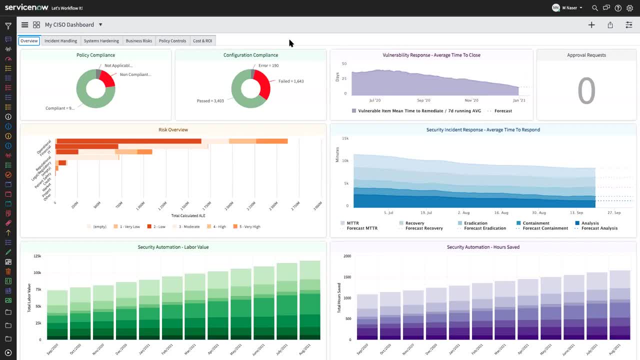 where we're basically going to be able to see an overview of the security posture within our organization. So from here we get to see what is the vulnerability response. what is the average time to respond to vulnerability Security answer response. what is the average time it takes us to respond to? 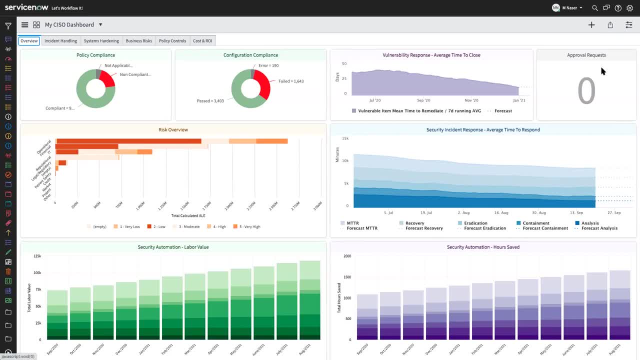 different security incidents. I've also incorporated the approval request and this is where we basically get to determine if the system needs to attend to any specific request or approve them, reject them, send them to review, etc. We have different tabs over here, which helps us dig deeper into different 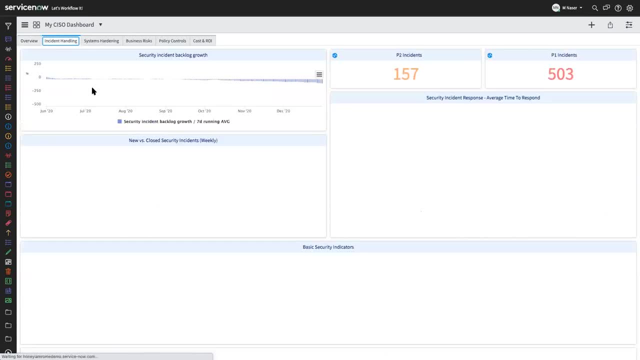 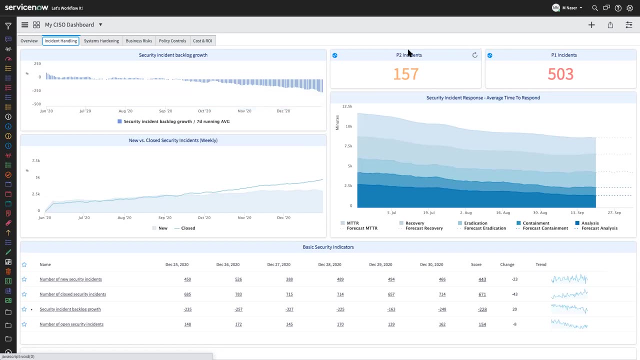 areas. So, for example, if you want to dig into incident handling, then we can see how many security incident backlog growth we currently have, how many priority one versus priority two incidents we are currently working with. We can see the security incident response. what is the average? 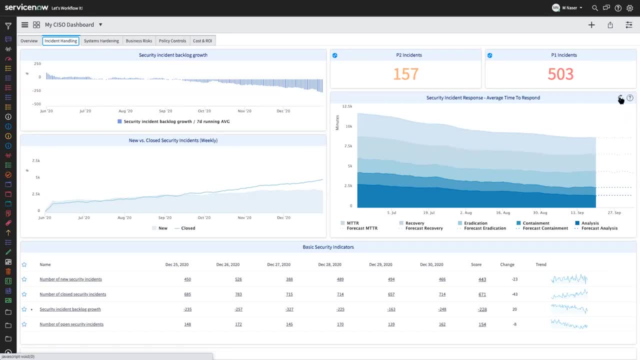 time it takes us to respond to different security incidents. To get the latest information, we can just quickly refresh the graph. We can also interact with this graph. So, for example, if I want to filter out the information or add it back in, I just click on it. and hovering on the graph, 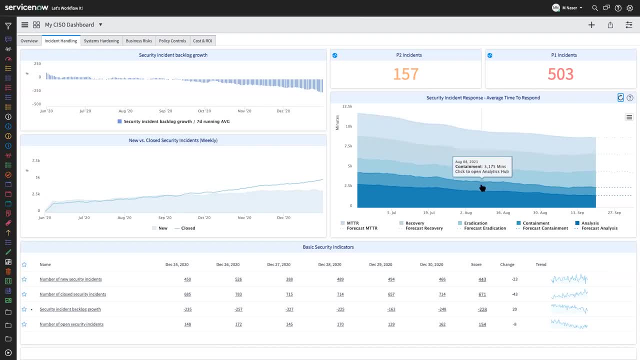 would promote me to actually click onto any of these different areas to dig a little bit deeper and get more information. came in affectionately. So I have three players right now and one in the information about. so, for example, in the containment part, i can just click on it. 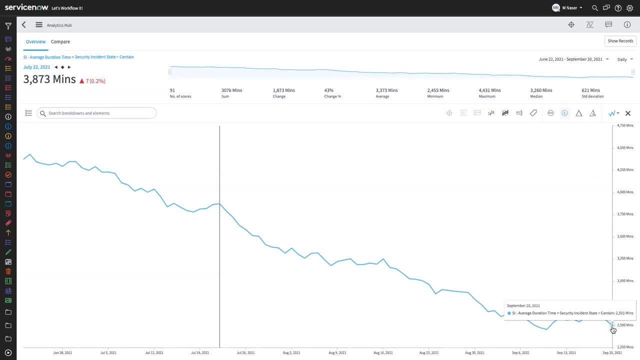 which shows me down to the minute what is our current performance when it comes to the containment. i can turn on the labels, which kind of gives me a better view into that. so it looks like we actually improved by one minute between here and the current time. if we want to create maybe a target or an initiative for the future, we can just quickly. 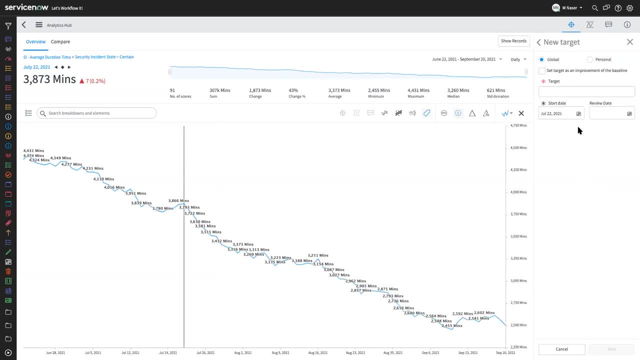 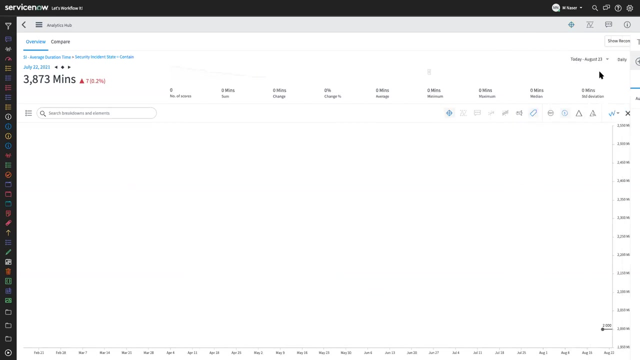 do that from here, where i can go ahead and say i want to create a target that is going to cut down the time to 2000 minutes by maybe july or whichever month i already get to determine. now, if i go back into my slide, i can actually check the target to. 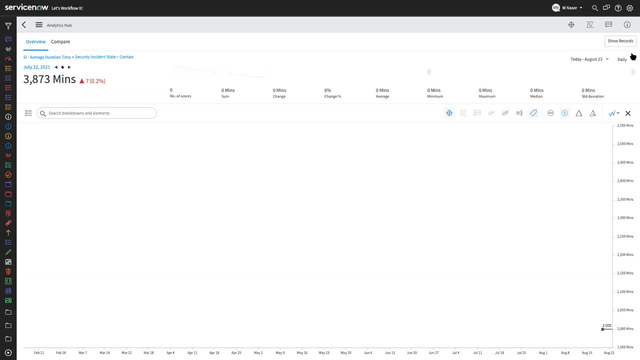 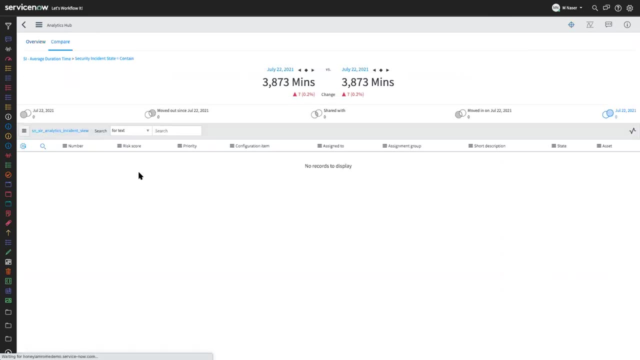 make sure that i am working or working toward achieving the specific target that i have created. obviously, here, on top of that, i'm able to perform or compare my performance between specific period of time. so if i want to compare this quarter versus last quarter or this year versus last year, 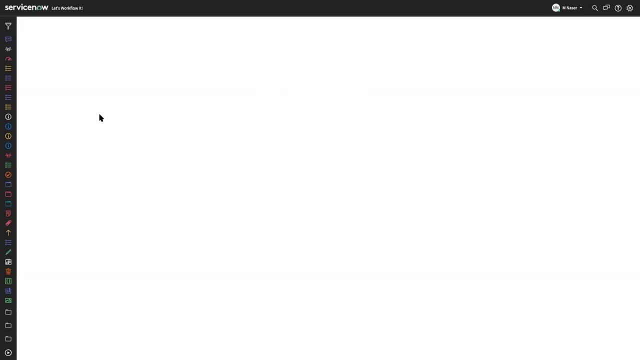 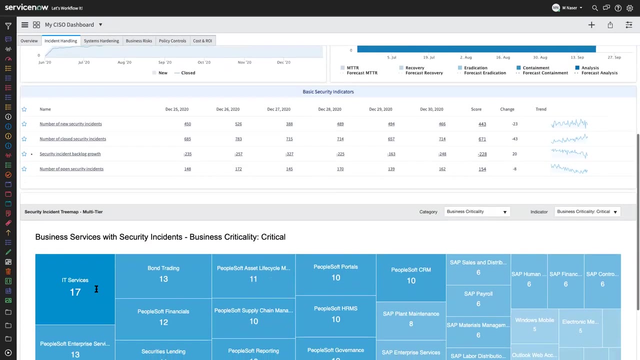 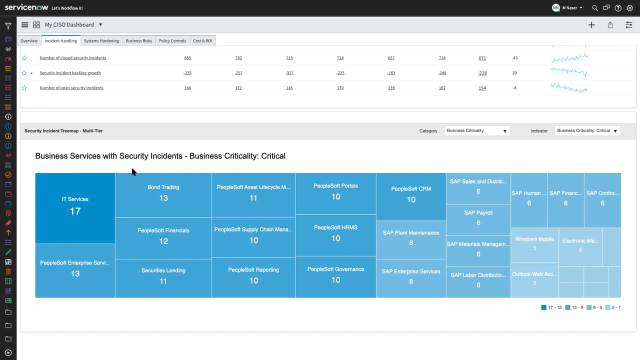 i can quickly do that right from here. uh, we also want to give the system the ability to make decisions on the spot, so i've incorporated the incident tree map over here, where we are able to look into the different security incidents that we have received, to understand in which department they rely or are in. so it looks like from this view, i can say that. 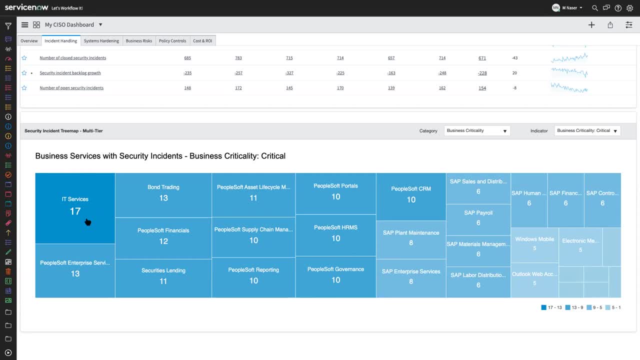 most of the security incidents that i currently have are an it service versus the peoplesoft hrms or the peoplesoft crm. so in this case i can just um hire more individual to work on the it service or move some of the individual and less work department like this app role into it service. 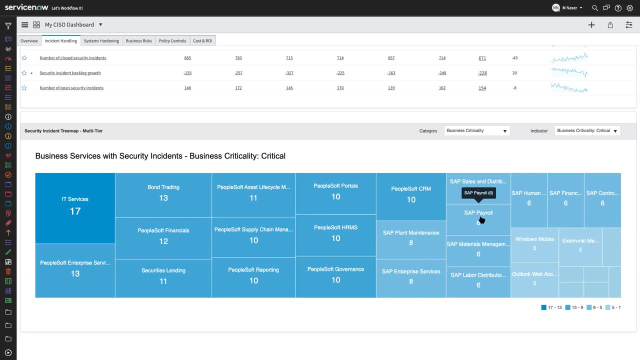 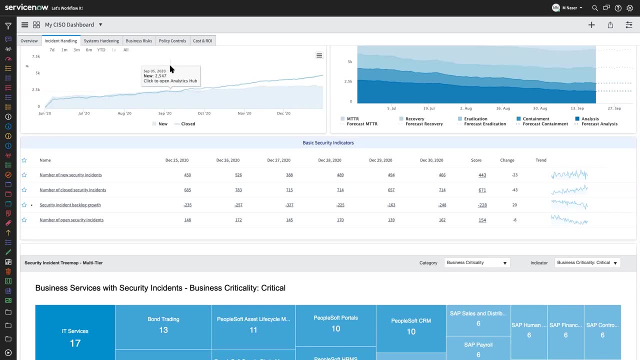 just to make sure that none of my teams are being overworked. now the next step is to make sure that the rest of the tabs over here are going to be digging into different information or different integration within the platform. so the system hardening is specific for vulnerability response. 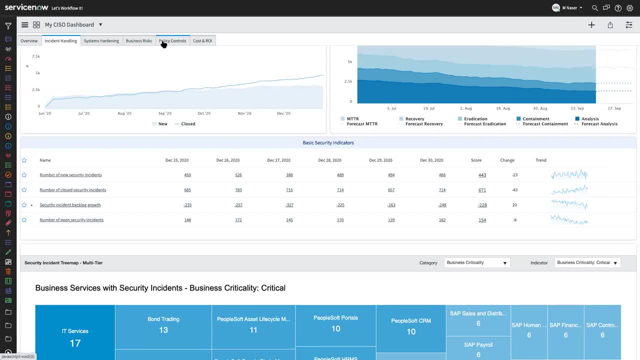 business risk and policy control are going to be something that is related to the integration with integrated risk management. another solution that we offer here at service now- cost and return of investment- is just a way for us to actually see the automation process that we have done on the platform and how many hours we've saved. 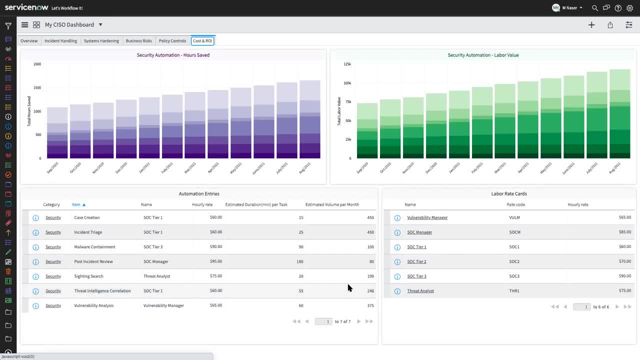 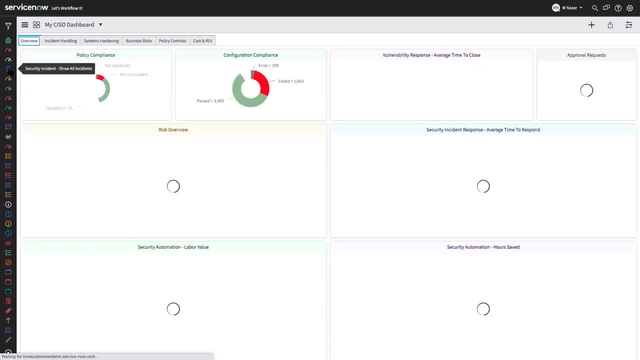 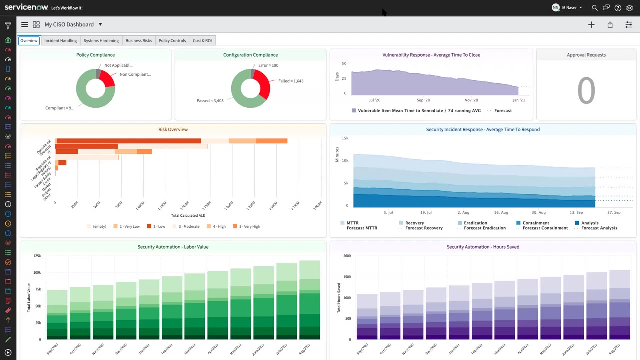 versus the labor value that we've saved, so this is something that is definitely beneficial to for us. so to understand the financial value of having something like service now implemented on their platform now moving on another dashboard that i wanted to cover would be the security operation efficiency, and this is kind of tailored to someone who is more in a management position to 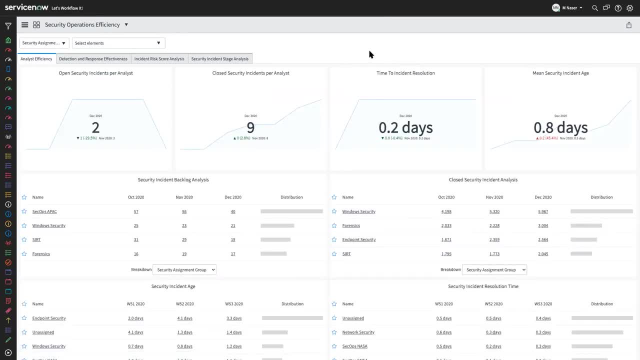 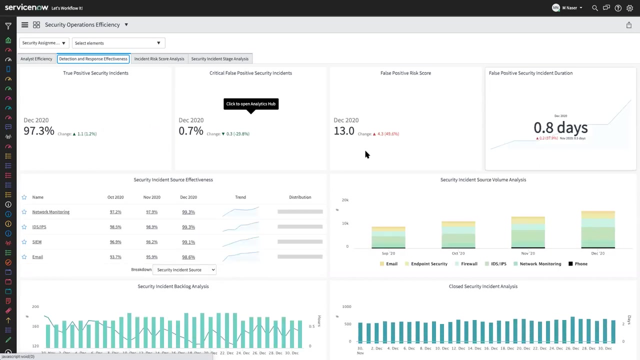 kind of understand: uh, what is the performance level of their team? so how many security incidents are there per analyst i currently working with? how many close security incident per analyst i can see the detection and response effectiveness for the different security incidents that i currently have. so how many false positives or score, how many false positive? 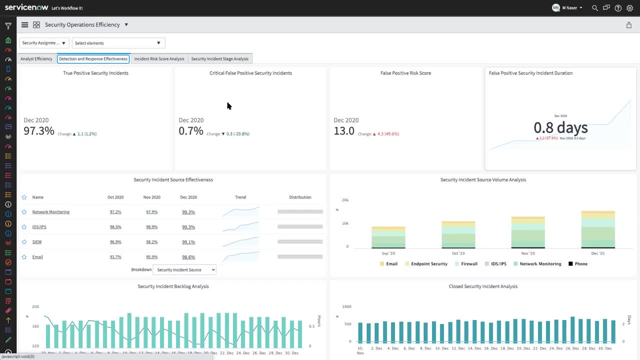 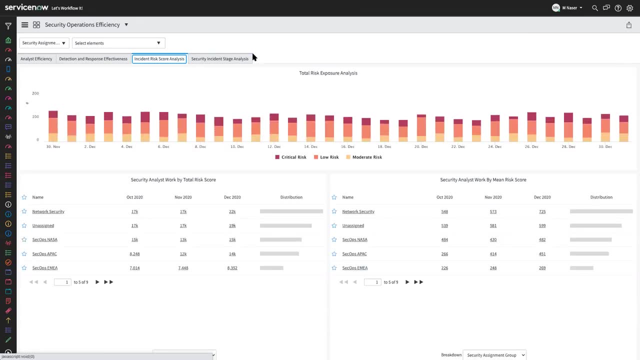 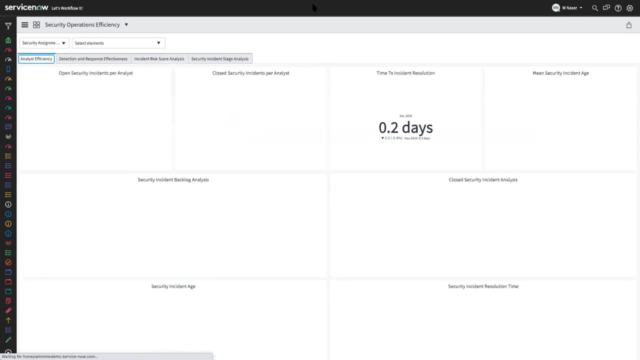 security incidents. what is the duration that they exist on my environment? the critical, false positive, true positive security incident, etc. i can see this in sorry the incident risk score analysis and the security instance stage analysis. so again, this is something that kind of tailored for someone who is in a manager position to kind of get more idea on their team. 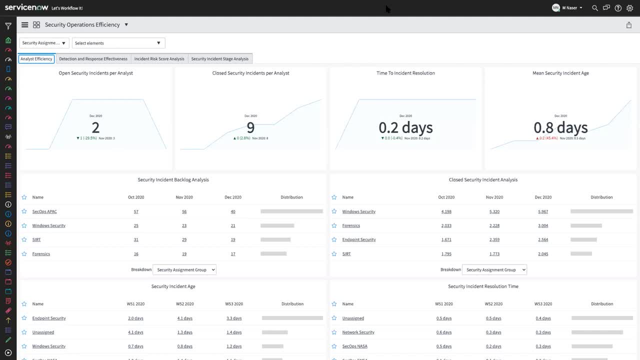 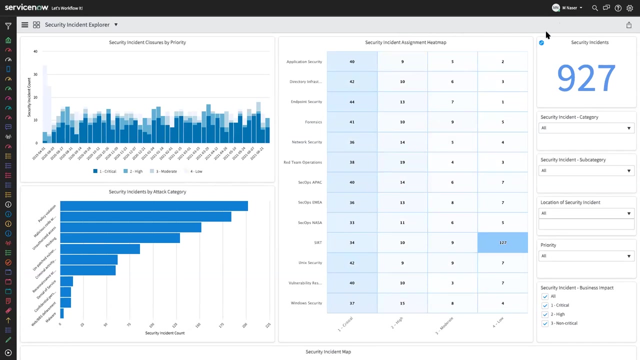 performance. now moving on to another dashboard, and this dashboard is going to be tailored to someone who is actively working on resolving these different security incidents. so, as an analyst, i can go ahead and see that the total number of security incidents i currently have within my environment is 927.. so the total number of security incidents i currently have within my environment is 927.. so this is another data set that i'm currently working on right now. 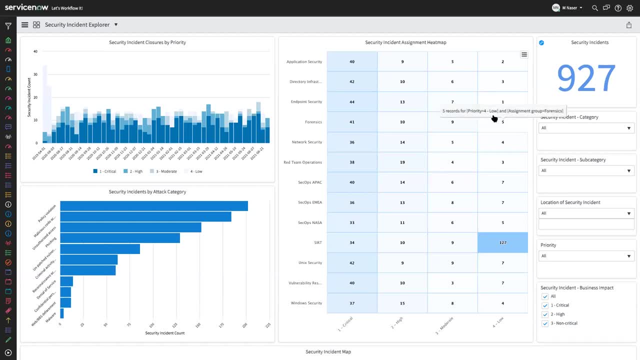 So this is a big number. This is something that is definitely gonna overwhelm me. So how can I get to know which out of these 927 I should be working on first? To do that, I can utilize the different filters that I have over here. 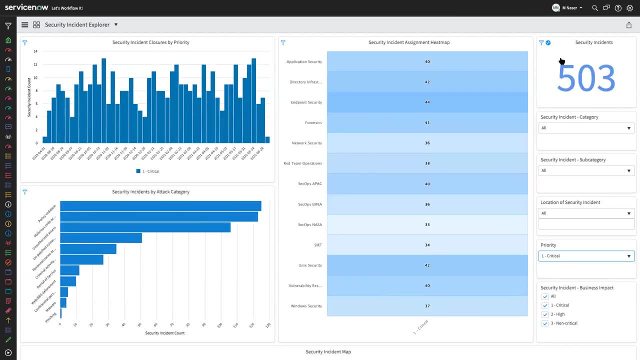 So I can focus on the ones that have a critical priority. So I can see how I immediately cut down the 927 to 503.. Furthermore, I can focus on the critical business impact to cut down that number to 450.. So with just quick filters I was able to cut down. 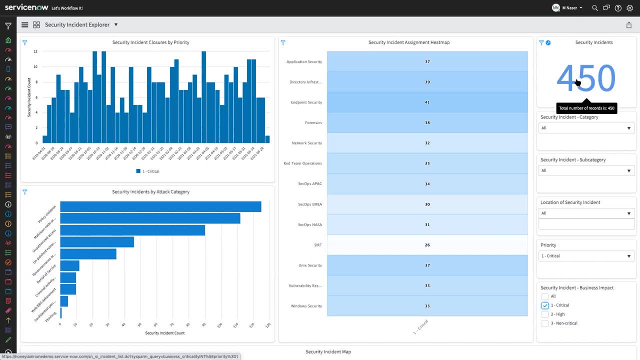 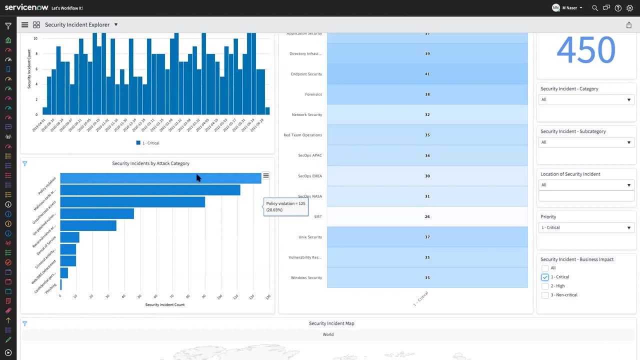 the number of security incidents that I should be focusing on by more than 50%. Now, out of all of these 450 security incidents, what is the security incident closer by the different priorities? What is the security incidents by their attack category? So, out of those 450, I have X amount. 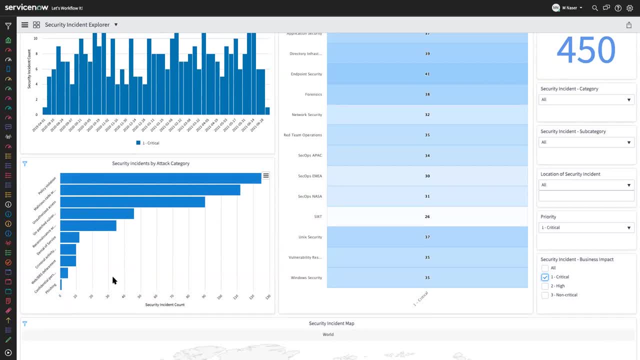 that is, policy violation versus denial of service, versus phishing. So this puts me in a place, as an analyst, to go back into management and tell them. by the way, most of the security incidents that we're receiving of a critical priority and a critical business impact are due to policy violation. 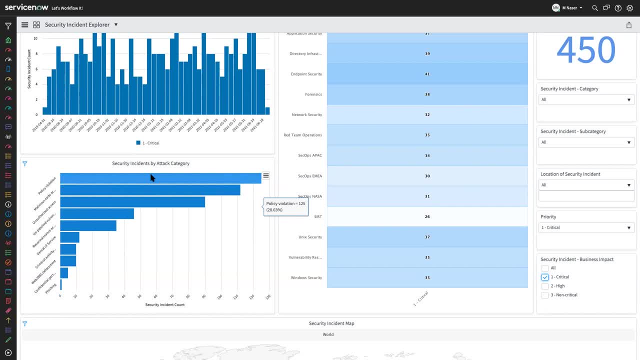 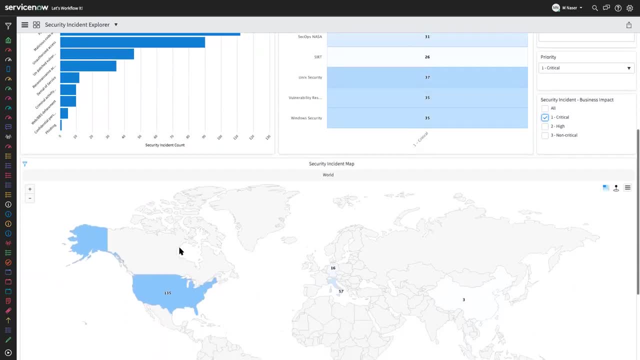 So maybe that puts us in a place where we need to train our employees more, or maybe enforce a better policy to make sure that everyone is adhering to it. Another thing that we can utilize is the visualization of the location of the different security incidents that we're getting. 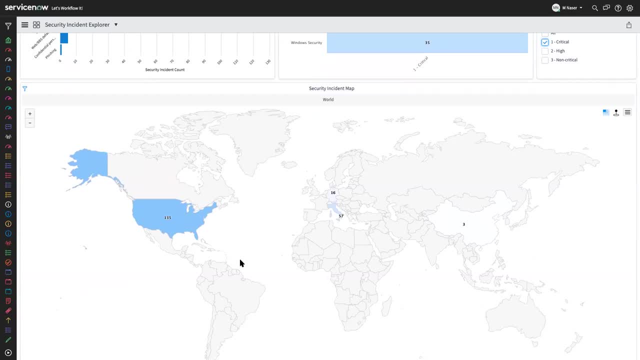 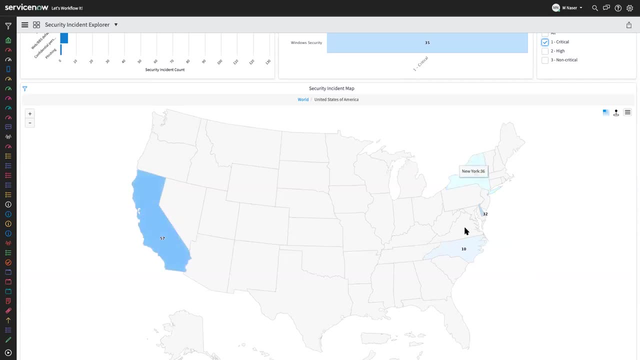 So I can actually look at this map and see how many security incidents are coming from where. So within the United States I have different offices. Some of them are in California, Some of them are in New York, Some of them are in North Carolina. 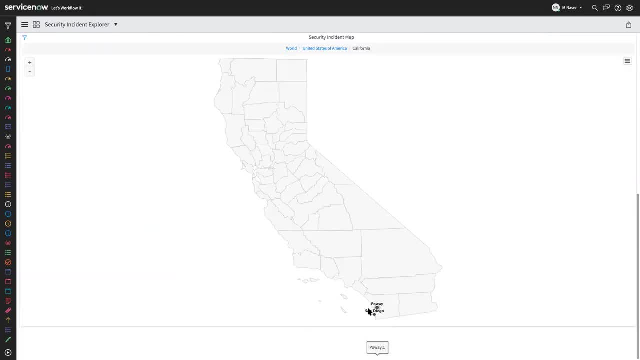 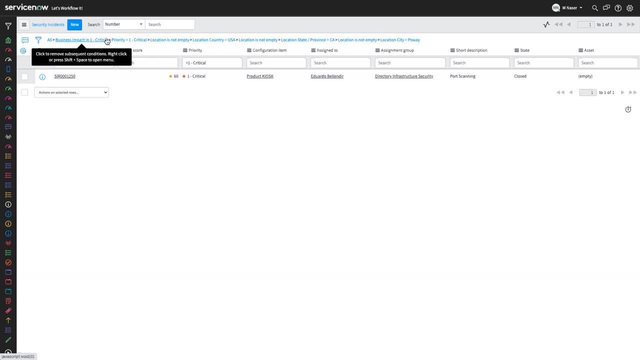 If I wanna focus on one of them. in my case, I'm actually located in San Diego, So I'm gonna be accessing this list, which shows me how many incidents that I currently have that have a business impact, that is a critical, a priority that is critical, that is located in San Diego. 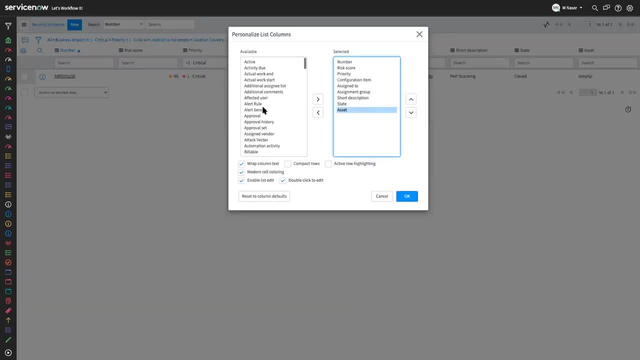 This list view can be modified if I wanna add in any information, like if I wanna see who is the affected user in this case, or if I wanna remove what is the short description for the security incident. All of that is immediately going to be updated. 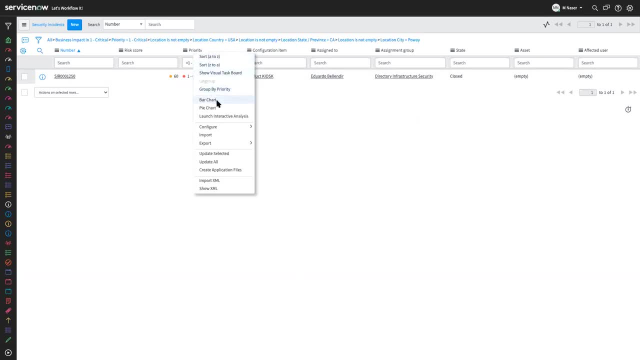 on this list view. I can do things like creating different reports for bar chart or pie chart of the different risk score. If I have more than one, in this case, I only have one. I can also export this graph that I created into any of the dashboards that I have access to. 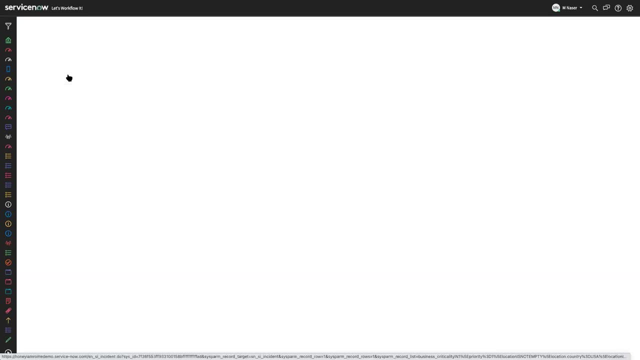 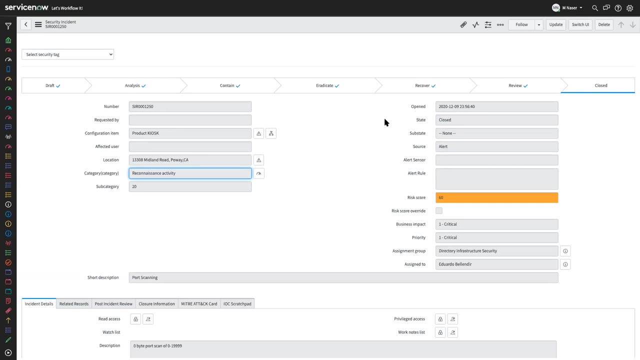 Now let's click on this security incidents to see how the security incidents and then trick it looks like. So over here on top we can see the different states that the incident had gone through. So in service, now out of the box, we follow a list stateful. 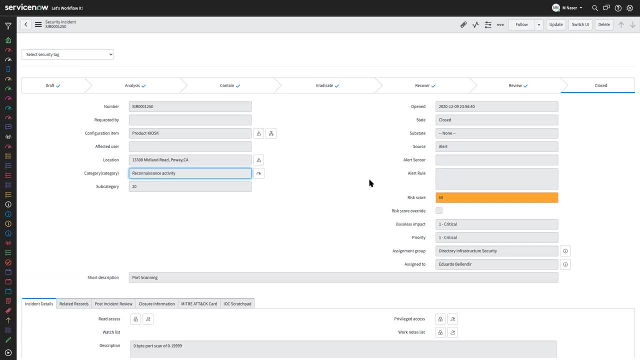 So the draft analysis contained for the case recovery review closed as all out of the box. And if your operation actually utilizes a different approach, like the list open, or if you have your own specific states that you would like to modify, all of this can be configured once you are actually. 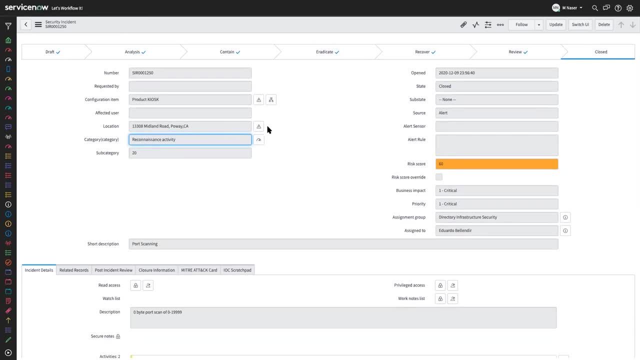 implementing the solution. Scrolling down into the incident record, we can see its number, who requested it. the configuration item: it's in location subcategory. We can see the risk score and the business impact and the priority. How did we determine this? 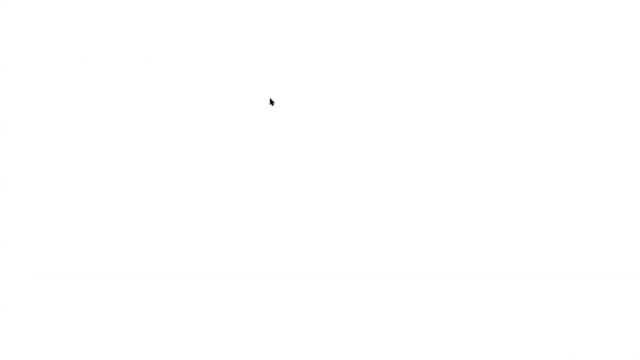 We actually did this through the CMDB. So if we open the dependency view map, we can tell that the security incident happened in the computer product kiosk. So based on what are the other services that can be be impacted if something goes wrong? 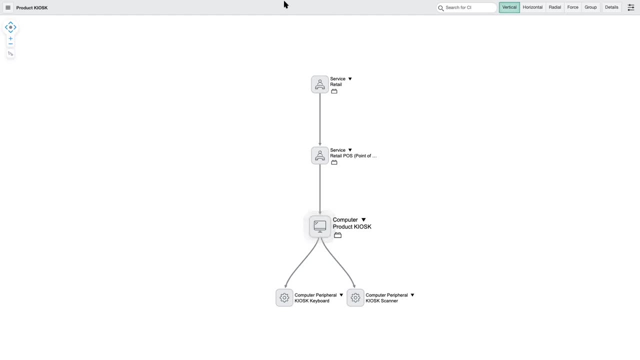 how critical these are to our operation. we can have the environment automatically associate the risk score and a priority for it, In this case, the risk score and the priority, that's where determined is 60 and the critical business impact and the critical priority. 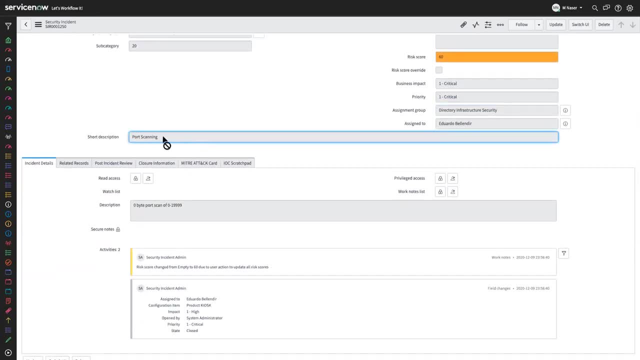 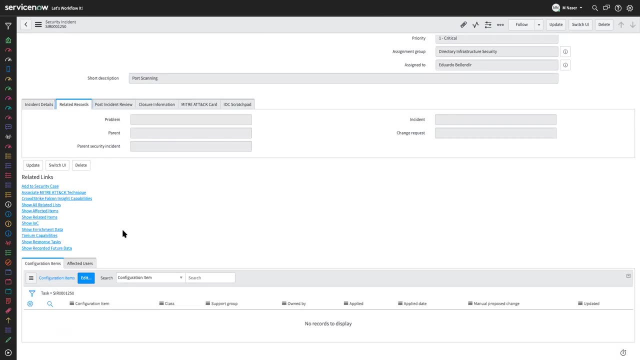 Scrolling down we can see a short description on the incident itself. We can see the incident details reported over here. If there are any, any related records in ITSM, for example, like an incident, a change request or a problem. 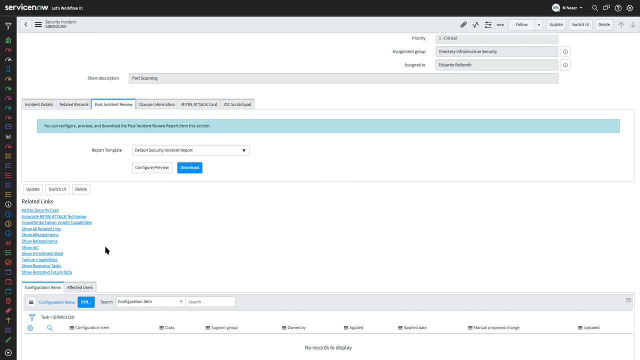 all of these are going to be available to me here. Post incident reviews again. this is where we're going to be basically sending out assessments that explore, check to see who had worked on this incident. What are the tasks that they have done? 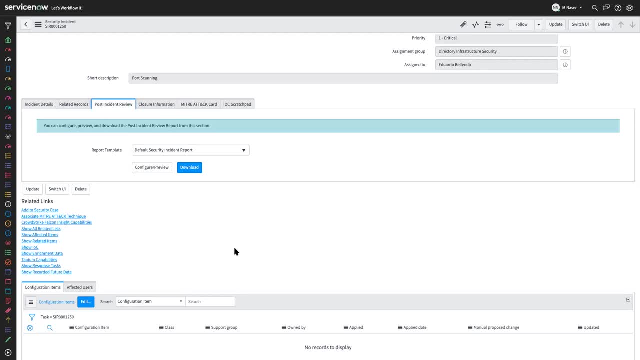 We can ask them specific questions that can help us into remediating this sort of incident in the future. We can utilize this to build a playbook in the future, or we can improve the current playbook that we used to resolve the security incident. 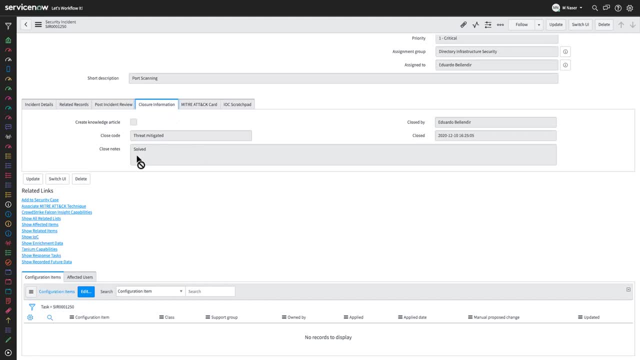 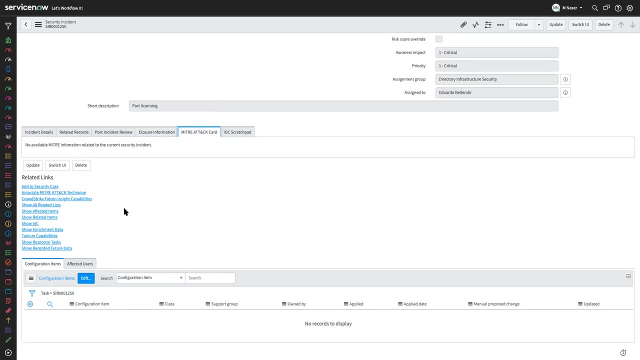 Closure information. This is where we keep track of when it was closed, What is the closed code, If there are any notes associated with that, This is where we can utilize the MITRE ATT&CK to see if this is part of a bigger technique. 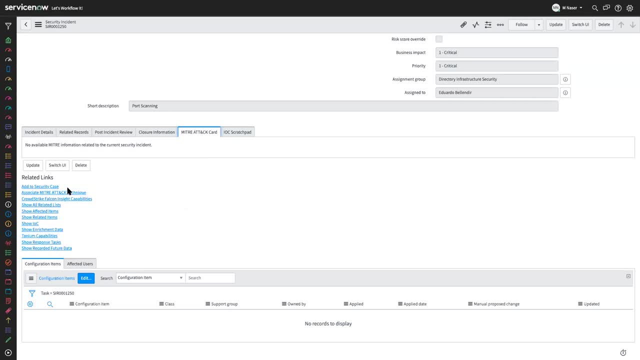 that we're not aware of or we should be aware of. Over here we have a bunch of different related links and related lists. It's like, for example, if we want to see the indication of compromise, we can just quickly click on that link. 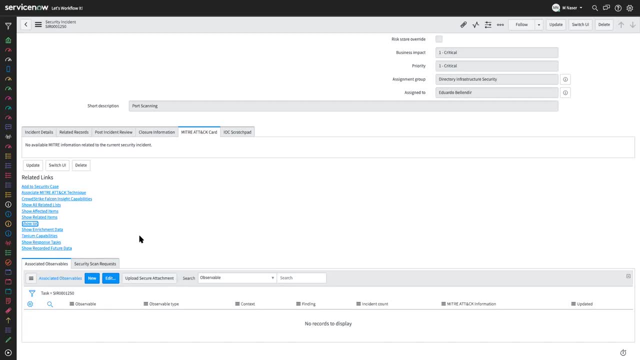 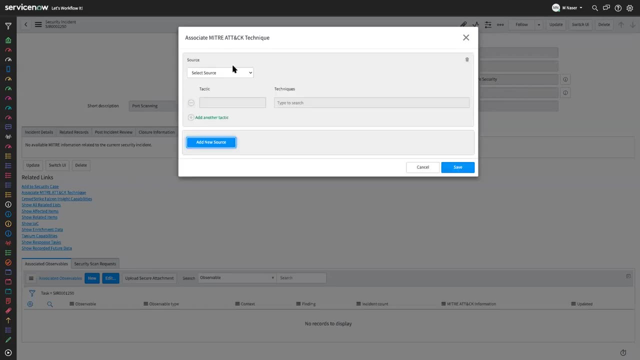 And if the information is available, it's gonna be available to us in the related tabs. We can associate this with a MITRE ATT&CK technique if we, based on our investigation, determine that it is in fact part of a bigger technique. 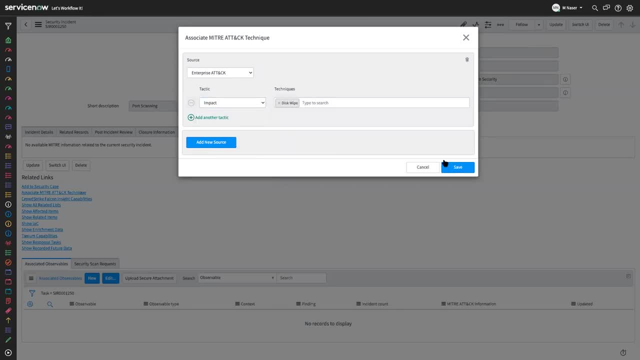 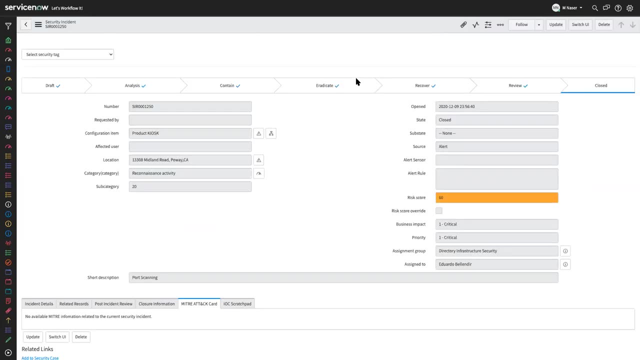 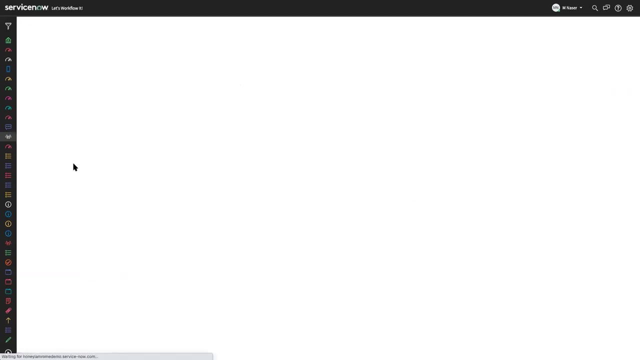 We can say that maybe this is an impact and a disk wipe just as an example, and then that would be reflected on the MITRE ATT&CK map, which I'm going to be covering toward the end of the presentation. So again, this is just a quick view into the incident record. This is an incident that has already been closed, So let's move on and actually work on a security incident from the scratch until the closure. 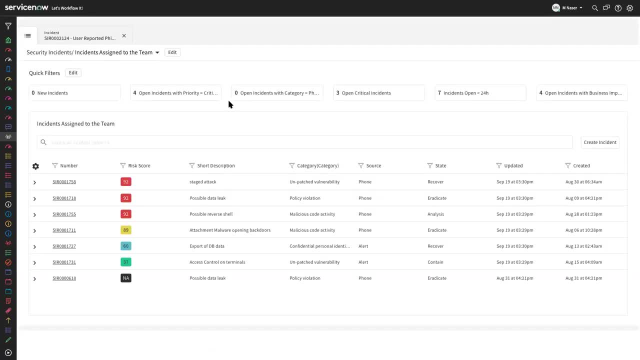 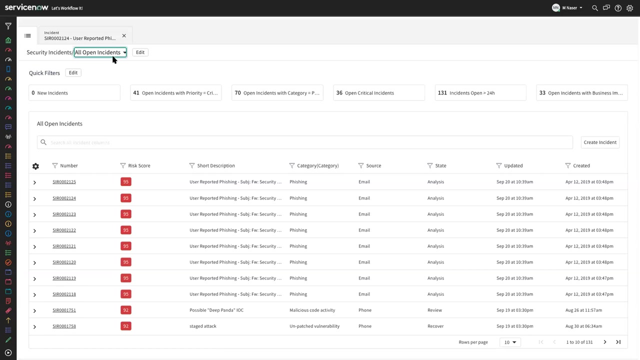 To do that, I'm going to be utilizing the Security Incident Workbench. So the Security Incident Workbench allows me to see all of the security incidents, in this case that are assigned to my team. If I want to change that and just look at all of the open incidents, I can just do that with a click of a button. 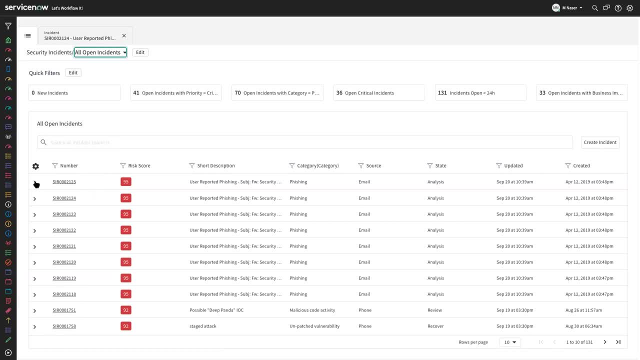 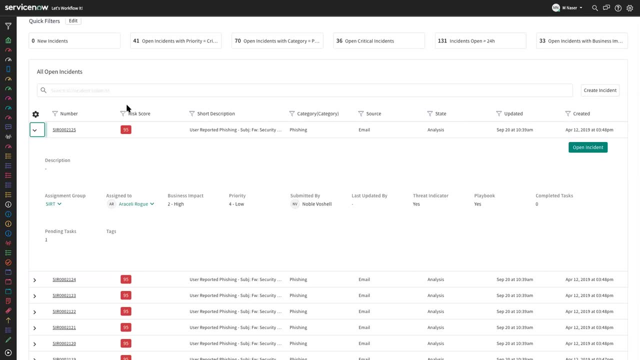 And from here I can get more information about the different security incidents by simply clicking on the peak view. So, as you can see, I can get more information about the security incident And if I choose to work on it, I can just open the incident in a new tab. 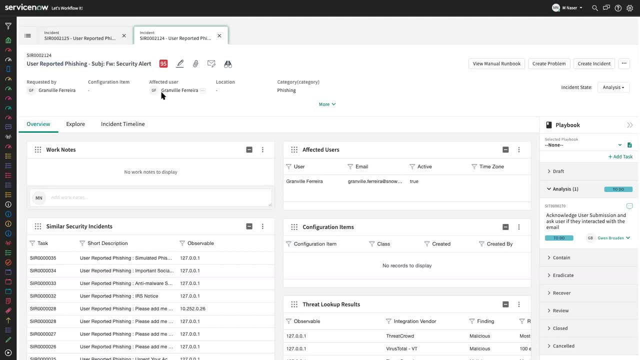 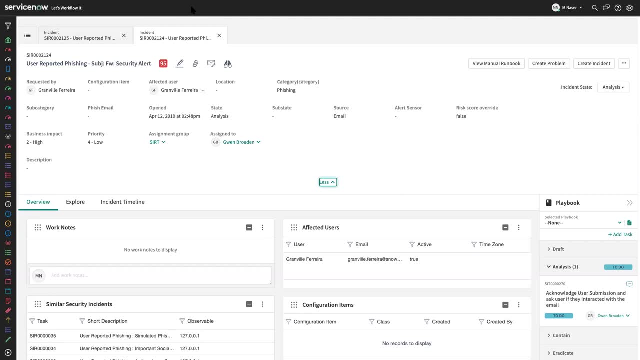 So over here I have two tabs for two different security incidents. If I click on more, I'm basically just going to be previewing, So I can get more information about the security incident, Like, for example, who requested it, the affected user, the category it's in, it's phishing. 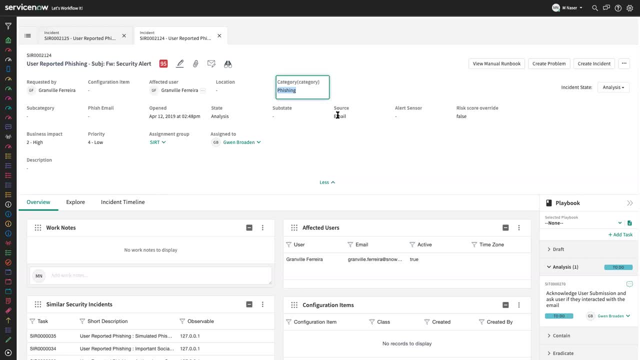 So as soon as we received this specific alert- and the source for that was through an email, So the user received an email- the click on report phish and the workflow for phishing kick in, which automatically pulled in the playbook for phishing. 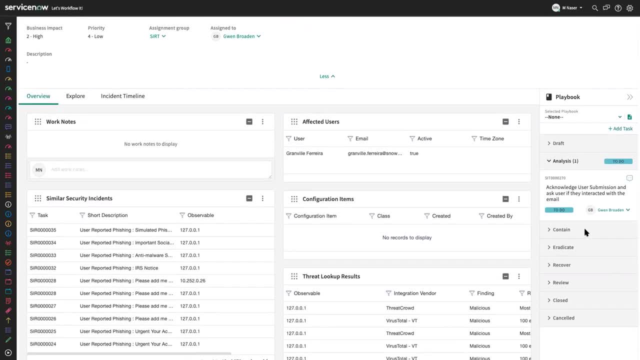 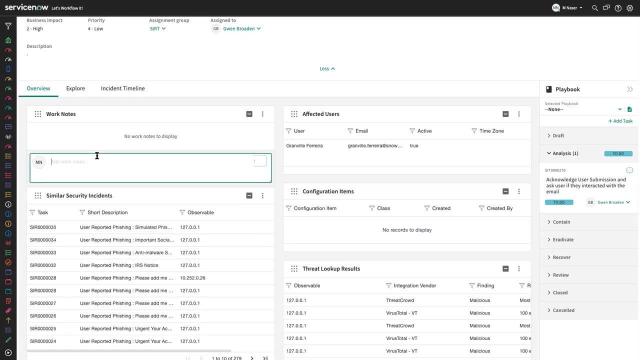 which gives us the appropriate steps that should be taken to remediate the specific security incident. Okay, Scrolling down, we can see how many similar security incidents we have: the work notes. So, again, cancelling out the silos, I can communicate with the IT teams or the security teams right from here. 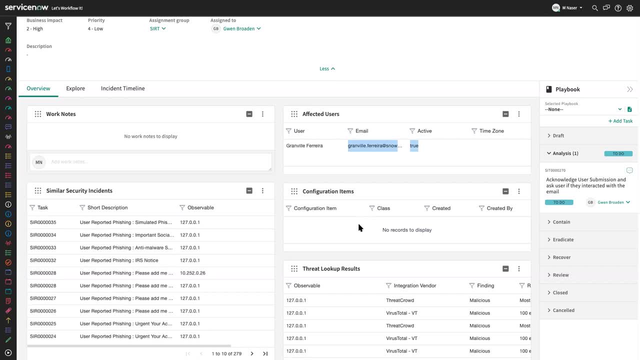 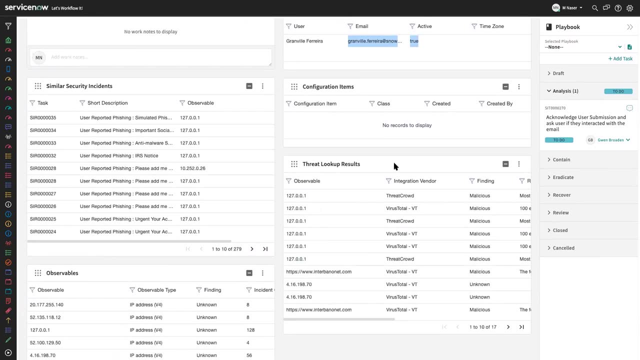 I can see who are the affected users, if there are any configuration items that I should be aware of or that are affected, And, before I even work on the security incident, I can see that the integration with ThreatCrowd and VirusTotal had already been taken advantage of. 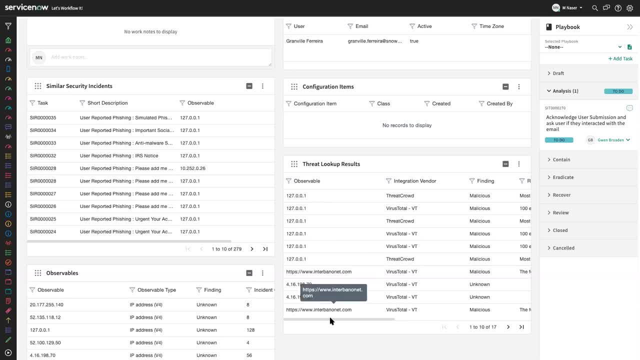 And we have seen how the IP address, the domain, if there are any hash attachments, have already been automatically scanned and we can see the findings for them. So it looks like this is, in fact, a phishing attempt and all of the information associated with it is malicious. 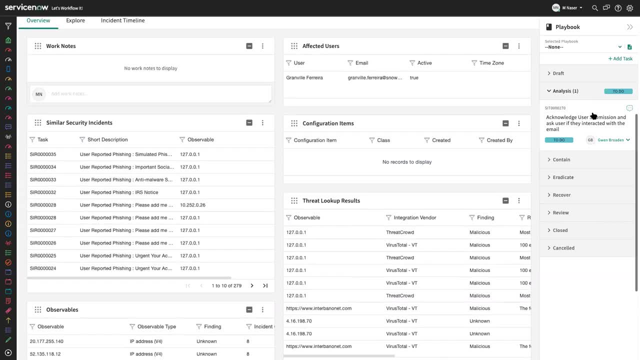 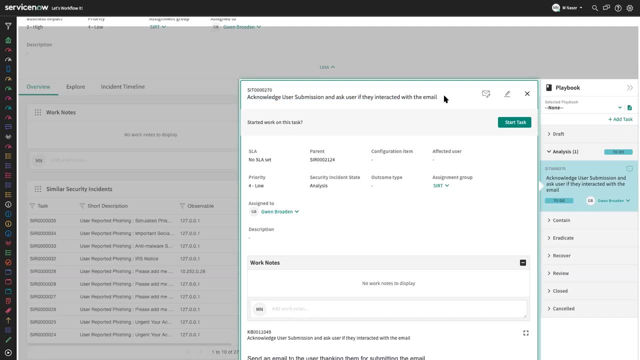 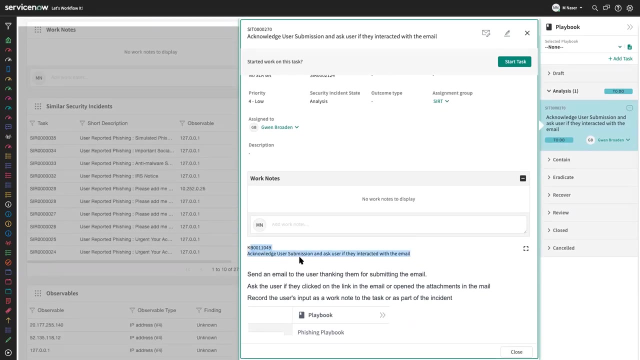 So let's go ahead and actually work on remediating it. So the first task would be to analyze it. How can we do this? It's to acknowledge the user submission and ask if they have interacted with the email. Now, if I am a newly hire and I don't know how to do that specifically, I can scroll down into the knowledge base article. 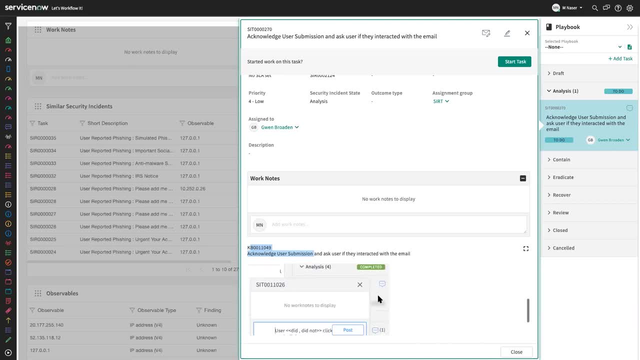 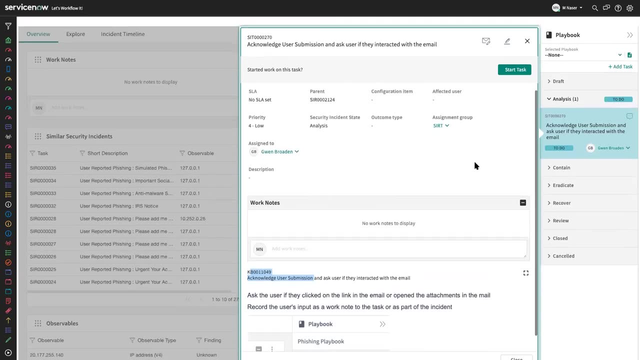 which shows me what exactly I need to be doing, down to how I should be reporting it back. So it looks very simple. All I need to do is send out an email Now. I don't need to leave this page to do that. 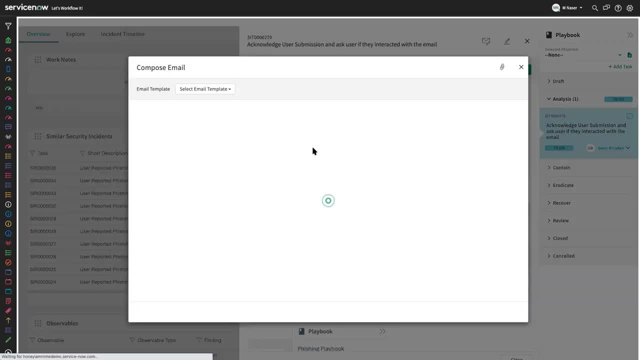 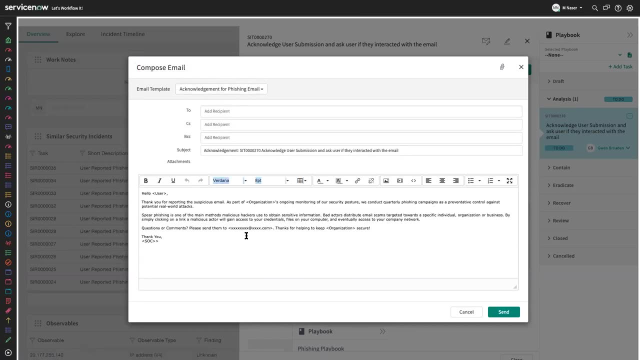 All I have to do really is click on compose email, Utilize the acknowledge for phishing template. I can see how the email is pre-populated for me. I can add in the recipient, change the title if I choose to do so, and send out that email. 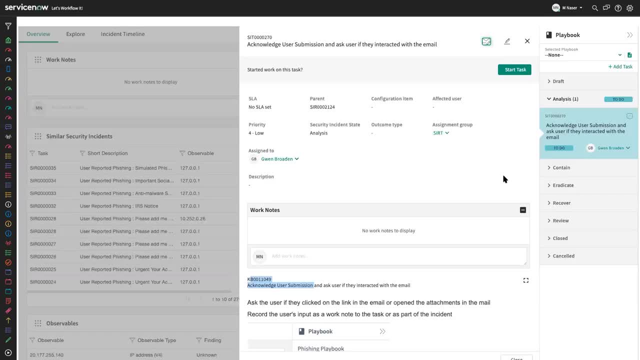 Now, while I'm waiting for the response, which can either be received back through a simple yes or no. this could also be sent out in a Slack message where they can simply click on yes or no. Based on the response, it could be reported back on my platform. 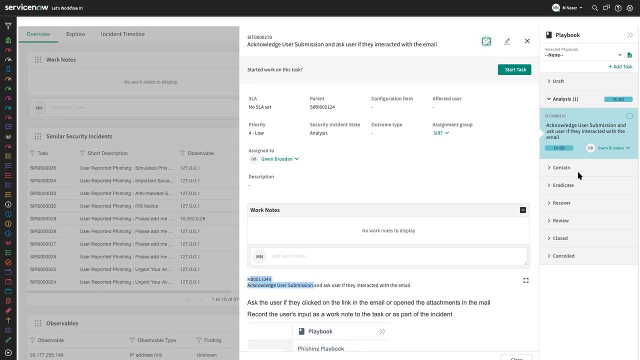 And based on the response- whether it was a yes or a no- the workflow can take different actions. So if they came back to me who were saying no, they haven't interacted with the email, then I can quickly close this as a false positive. 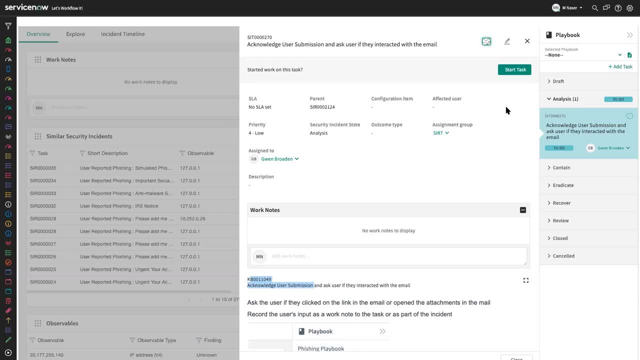 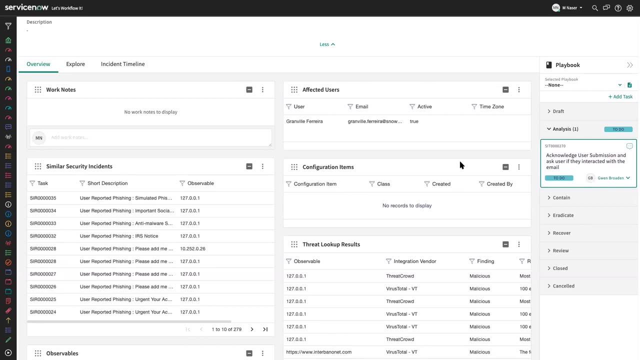 Versus if they came back to me saying that they have in fact interacted with the email, then in this case I am promoted to go ahead and isolate the host on how they have interacted with this email, just to make sure that if there is a worm or a virus, it does not contaminate the rest of our environment. 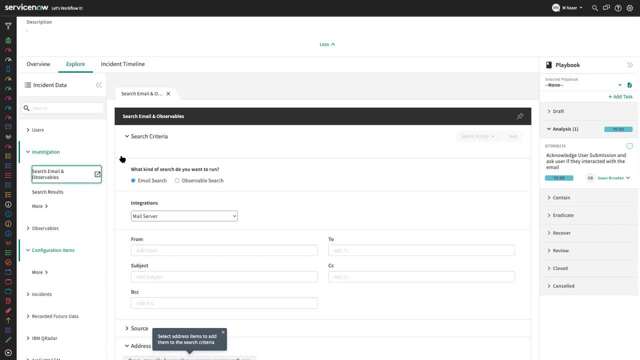 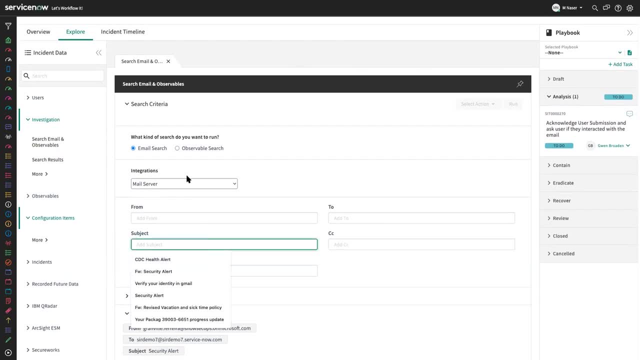 Now, while I'm waiting for the response, one thing I can do is I can search the email and observables for all of the email servers that I'm currently working in, So I can just look for the subject. So the subject was forward security alert. 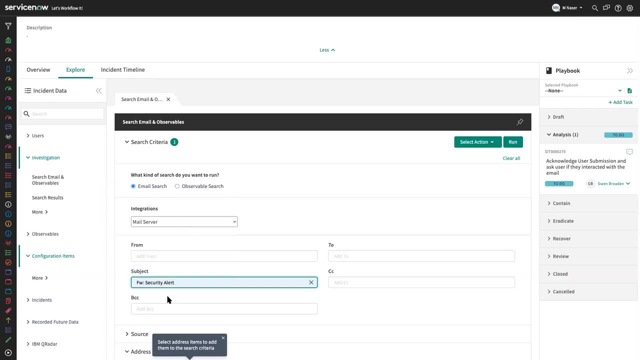 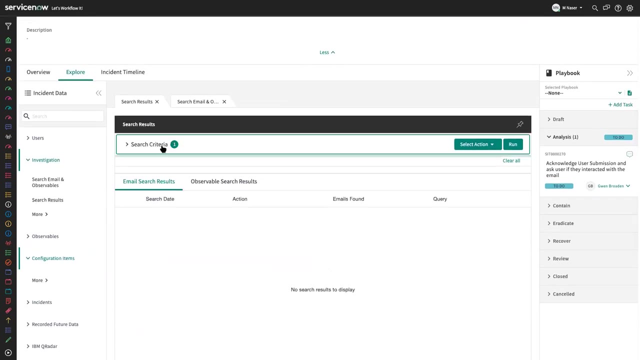 I can just go ahead here, say I want to look for all of the emails that have the subject within my email servers And I'm going to search. Just within a couple of seconds the search results come back to me saying that they could not find anything. 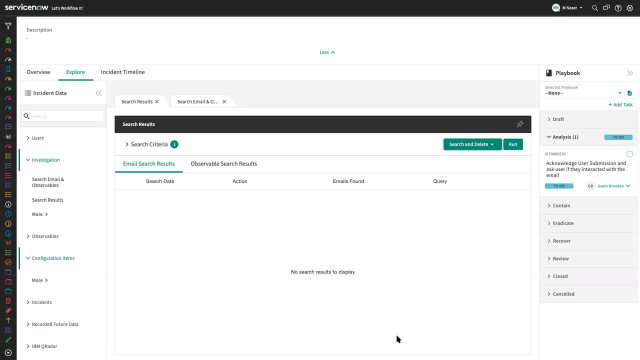 Now, in another case, I can say that I'm just going to search and delete because I don't want any other employees to actually interact with this email. Now, if the search had came back to me saying that there are more than one affected users? 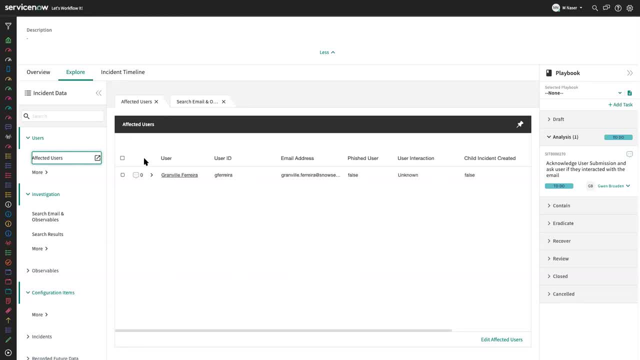 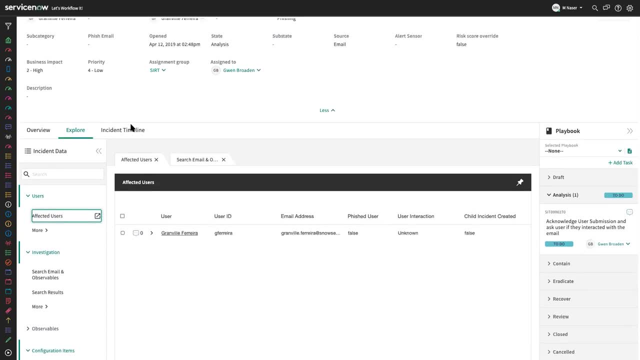 I can go ahead and see how the affected users are going to be automatically updated here, which means that the business impact and the priority are also going to be automatically changed. So in this case, since we have only one user who received this email, the business impact is high and the priority is low. 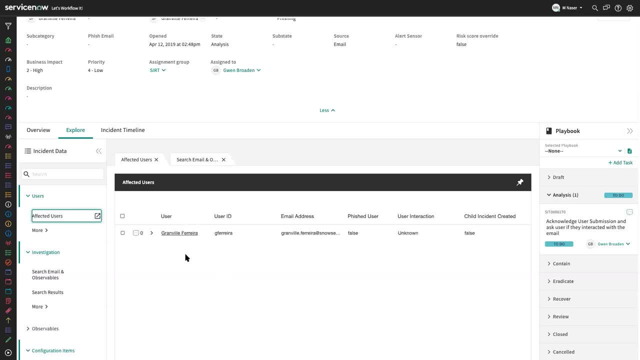 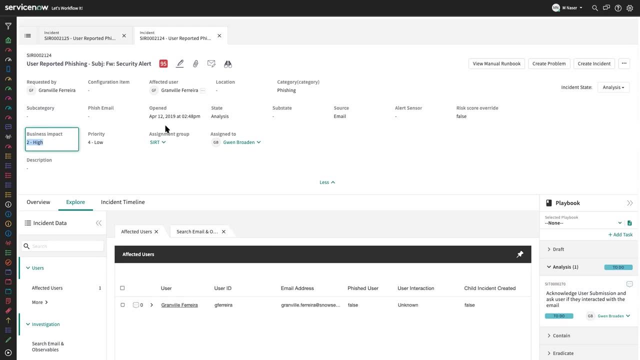 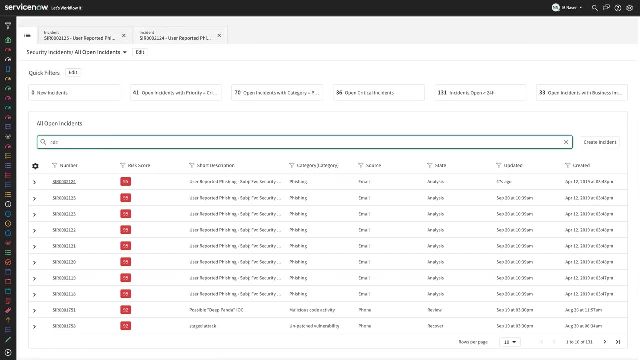 If the users stand into five or 15 or all of the organization, then the priority is going to become critical And the business impact is also going to be critical, Because all of the environment is potentially affected with this specific phishing attempt. To give you a better example of the search result, I'm actually going to look at a specific use case, which is the CDC. 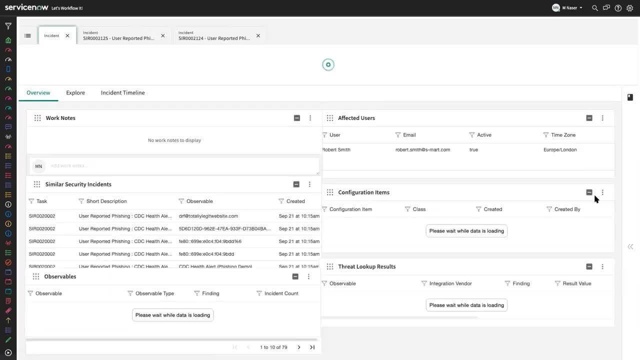 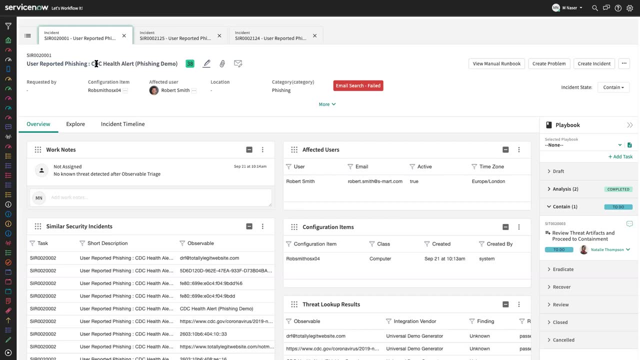 Again covering what we were seeing on these slides, how there has been a surge in the phishing attempts between March and April 2020.. So we created the CDC Health Alert, again just to show you how phishing can be done in this case. 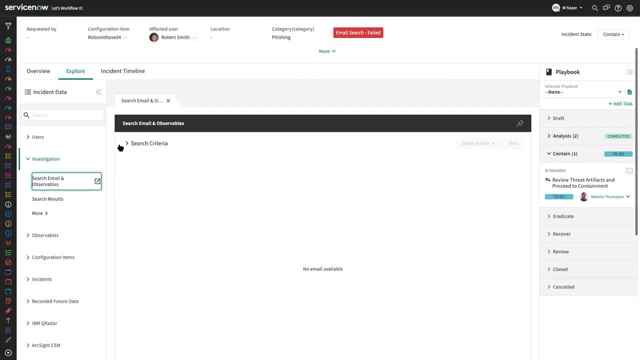 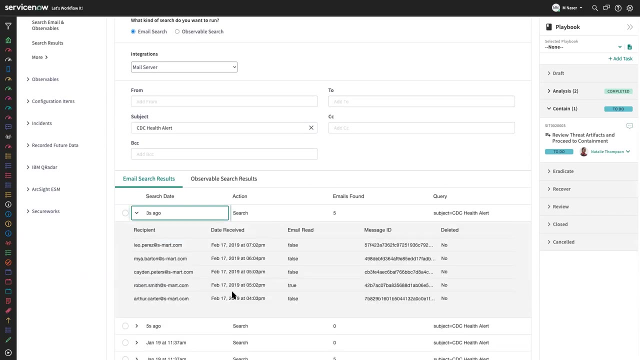 If I go into the investigation and search the email and observables for the emails that have this title, which in this case CDC Health Alert, I'm going to be actually seeing more information. So it looks like five individuals have received this email and one of them have actually clicked on that email. 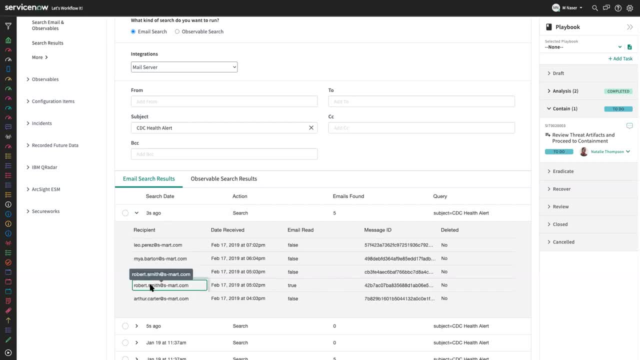 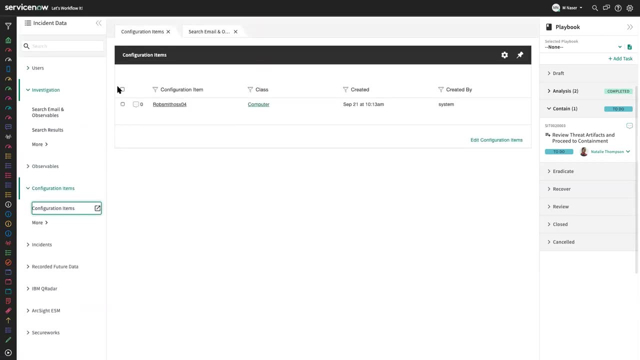 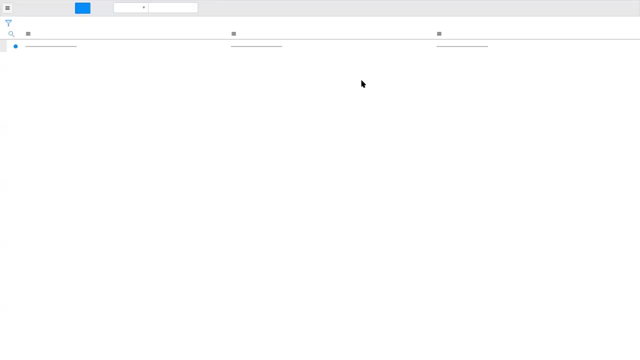 So there is a potential for an exposure, in this case from Robert. To remediate against that, I can go ahead and check the configuration items associated and isolate that host. Choose how I'm going to be isolating it through the Universal Demo Generator. 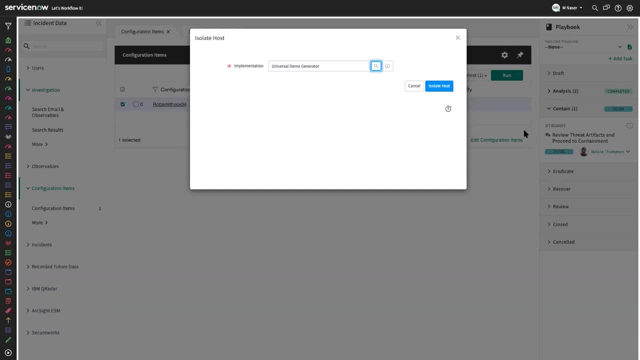 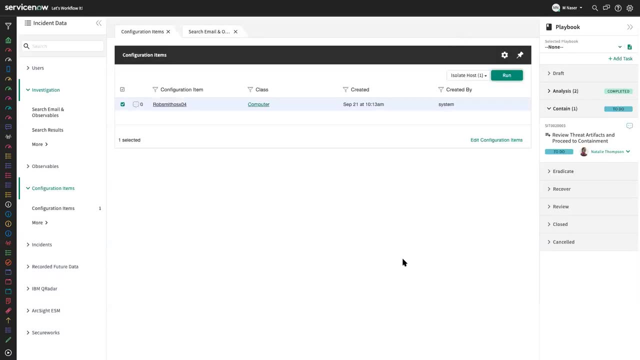 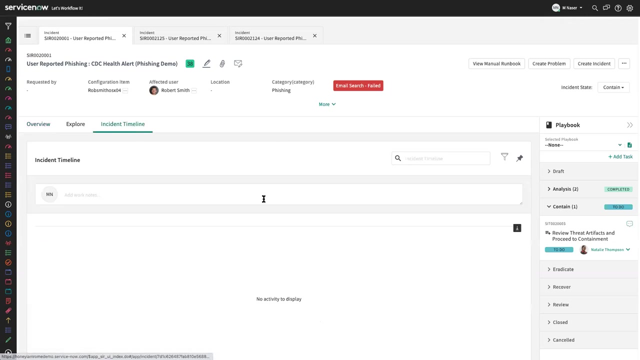 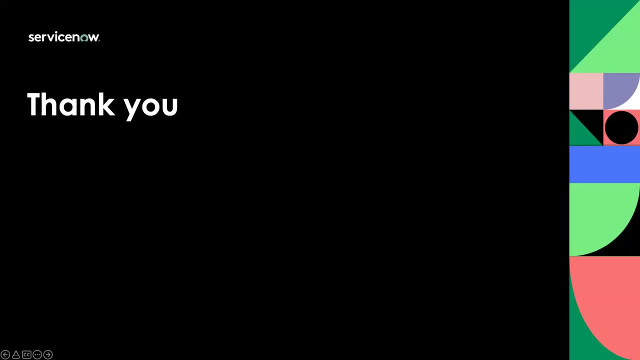 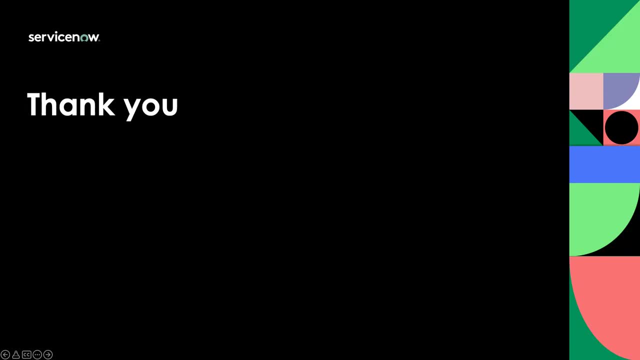 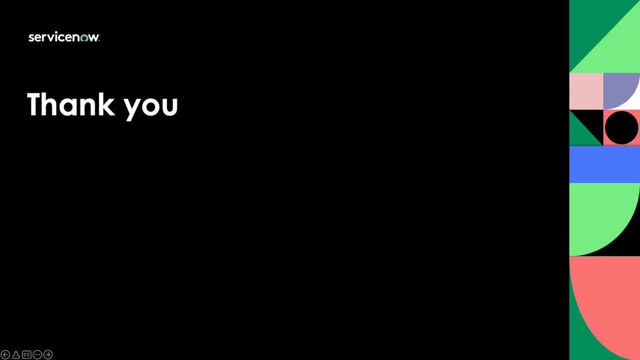 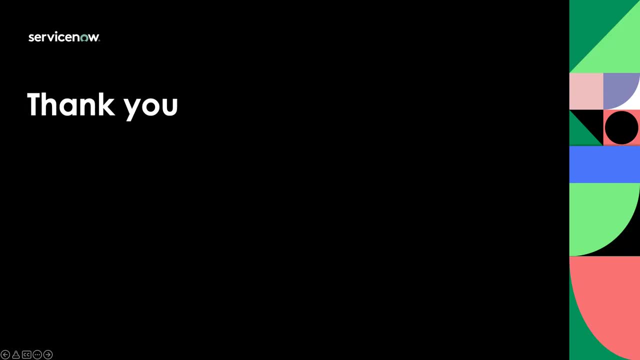 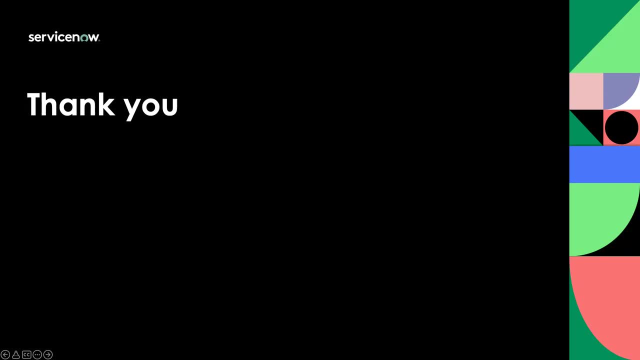